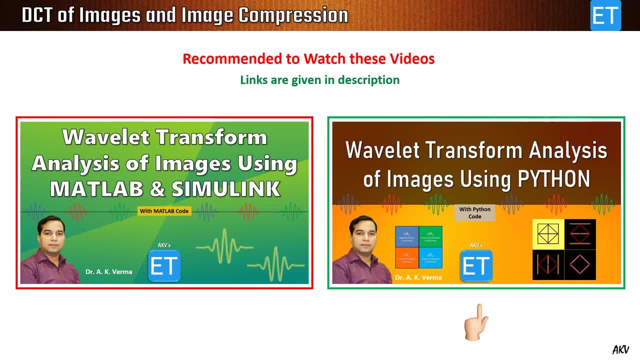 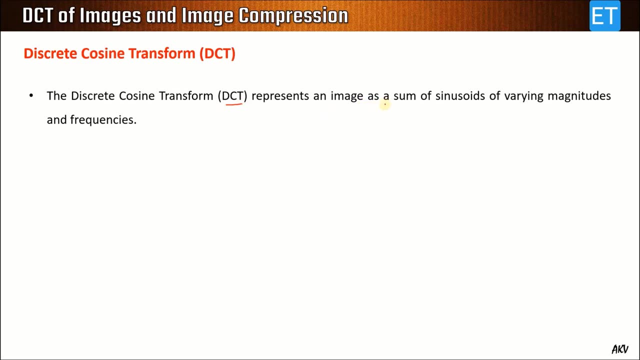 one is also the same, but it's implementation using python. These two videos link actually. you can find in the description. Now let us see what is discrete cosine transform. Actually, the discrete cosine DCT represents an image as a sum of sinusoids of varying magnitude and 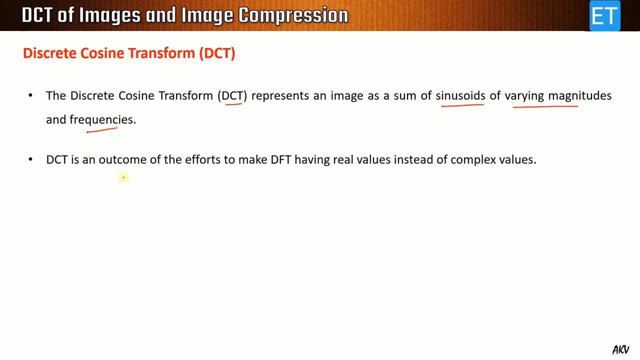 frequencies. DCT actually is an outcome of the efforts to make the DFT. DFT means the discrete Fourier transform, having real values instead of complex values. So the DCT, you can say it, is an equivalent of computing the two end points, DFT of a signal which is made even symmetric by its extension. So the 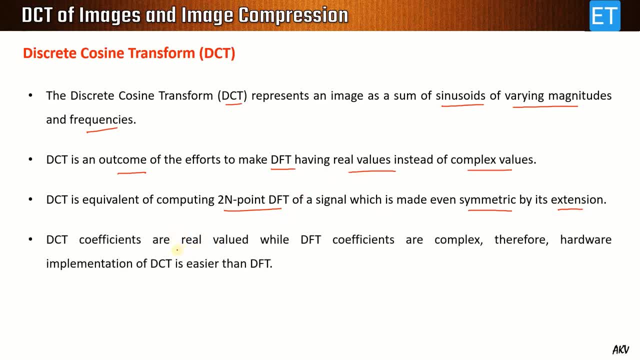 DCT coefficients as when compared with the DFT they are real valued. Therefore the hardware implementation of the DCT is much easier than the implementing the DFT. So also, if one can utilize the fast Fourier transform structures to compute the DCT, obviously it will be much faster computation. Therefore it has. 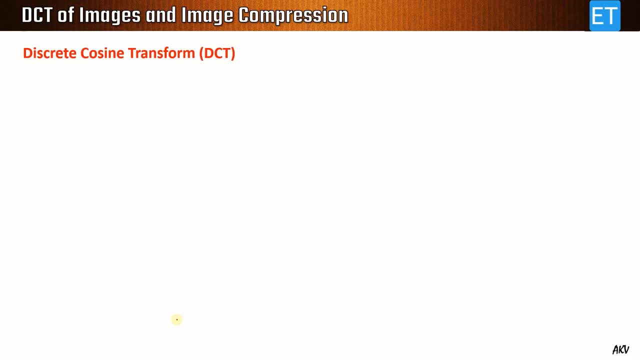 become the choice for many applications. The DCT actually has the property that for a typical image, most of the visually significant information about the image is concentrated in just a few coefficients of the DCT. So this property is known as the energy compaction property. Therefore, DCT finds: 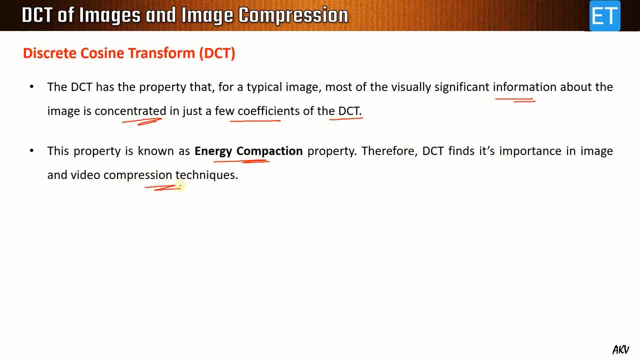 its application in image and video compression. So DCT is at the heart of an international standard lossy image compression algorithm, which is known as JPEG, which is very popular to represent image compression. besides this, DCT has actually the wise applications areas such as JPEG, as I already said apart. 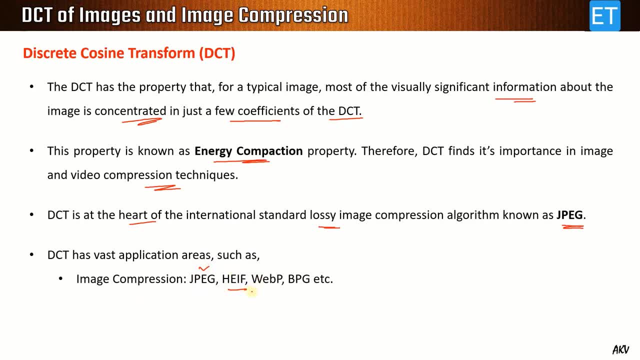 from this, it is found in HEIF, image compression, YP, BPG, etc. also, it is the main constituent of various video compression correct, such as h261, motion JPEG, MPEG 1, MPEG 2, h263 and then currently widely utilized h264, which is known as advanced video coding, or MPEG 4, and then h265, which is the latest one. 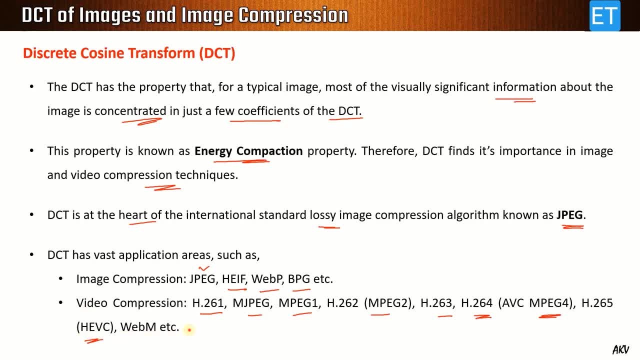 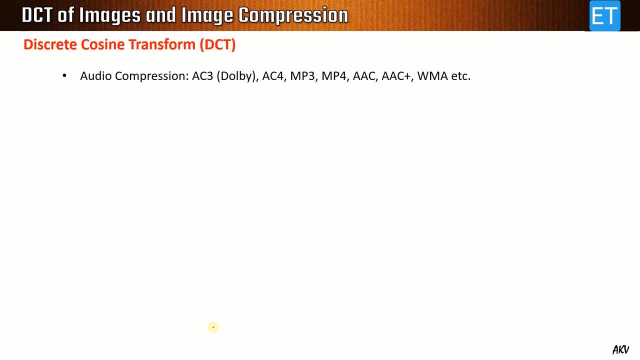 that is the high-efficiency video coding and then web M etc. various video compression algorithms, and it is also very popular in audio compression. it fine. it finds its importance in AC 3 format and modern AC 4 and it is a part of very popular mp3. 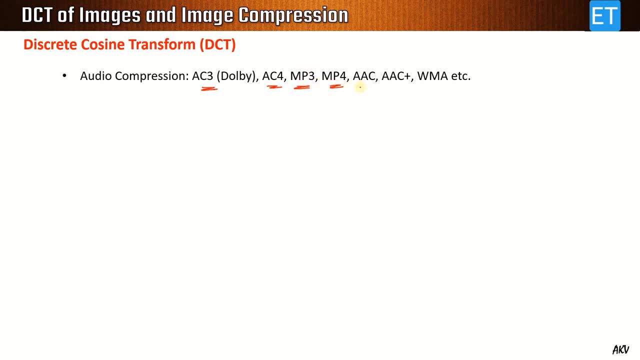 audio compression algorithm and before a AC, a AC plus and Windows media audio, etc. you can find the importance of the DCT in the speech coding, such as voice over IP, and in speech coding such as voice over IP, and in voice over IP and in the digital radios, and also you can, of course, solve a partial differential equation using the dct. 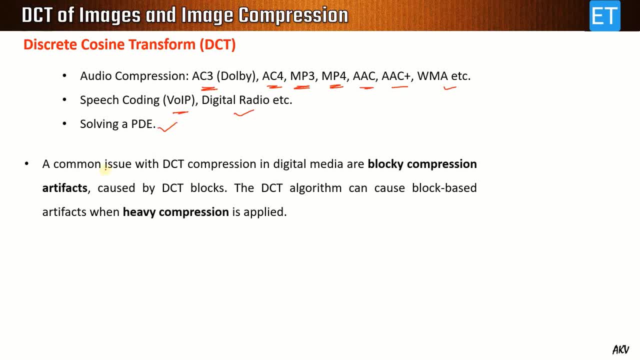 besides all these advantages, it has a few disadvantages also. for example, a common issue with the dct compression in digital media are blocky compression artifacts caused by the dct blocks. so the dcd algorithm can cause the block based artifacts when the heavy compression is applied. so in this image you can see- it's your jpeg image- when the heavy compression is applied. 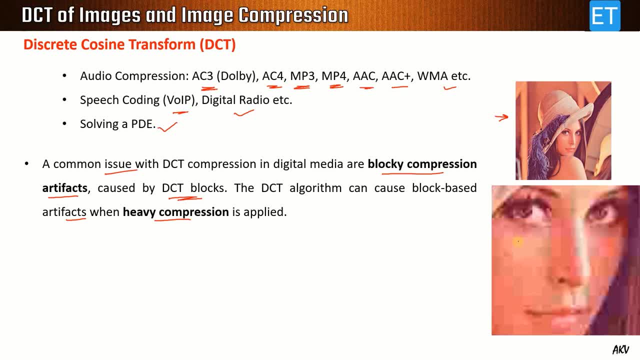 and after zooming it you can see that these, these are small square squared blocks in the face. you can see. so this is known as a blocky compression artifacts. so these actuallyuh in jpeg. these are small 8 by 8 pixel blocks. also, if you truncate the higher spectral coefficients in dct, they result. in the block dct decentralizedcionals. so if you just truncate that block they sink into the block size of dct, which only accounts for that expressed activity. so you could be possibly able to discover the basic rules of block dct alpha go, the promise that this bar is possible. um, a samples if i'm out of the digital. 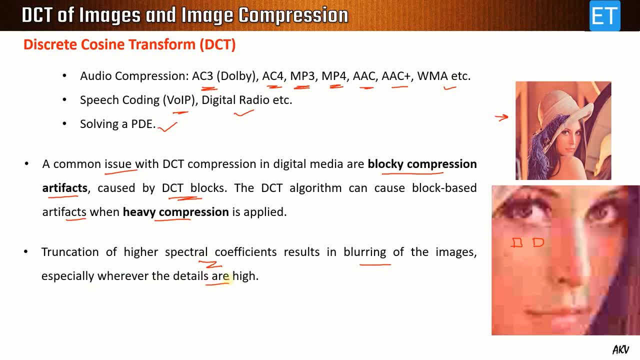 blurring of images, especially where the details are high. and if there is a quantization of the low spectral coefficients, they introduce the graininess in the smooth portion of the images. so these are few disadvantages of dct in image and video compression. now let us see how we can. 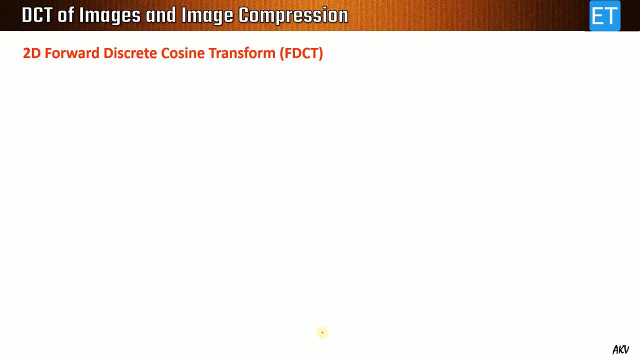 find the two-dimensional forward discrete cosine transform of an image f x- y having size m by n, so that you can achieve, using this equation to question one: so this is your image f x- y and here it is multiplied with these two: cos cos pi two x plus one, p upon two m. cos pi two y plus one. 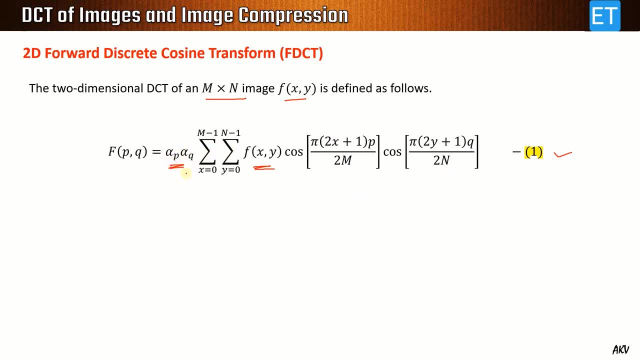 q upon two n, and these are two coefficients, alpha p and alpha q. so, after implementing this equation, your f x y is converted into a matrix- f p- q- that is equivalent in the size of f x y and it is carrying all the dc2. q is equal to q, x and y is the number of coefficients you need to be able to. 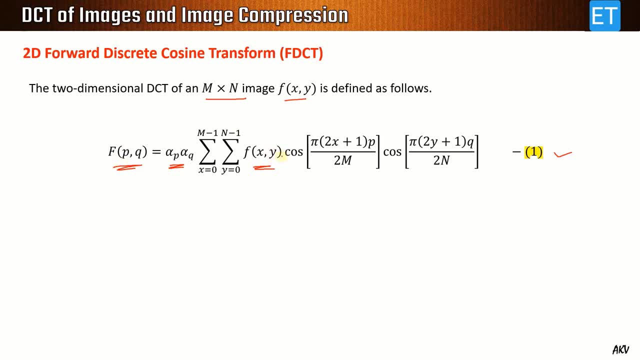 calculate the length of the image f, x, y and m by two so you can get this equation and here in image coefficients. So this equation you can implement in software by writing four for loops, The two for loops actually for the p and q, where p is varying from 0 to m minus 1 and q is varying. 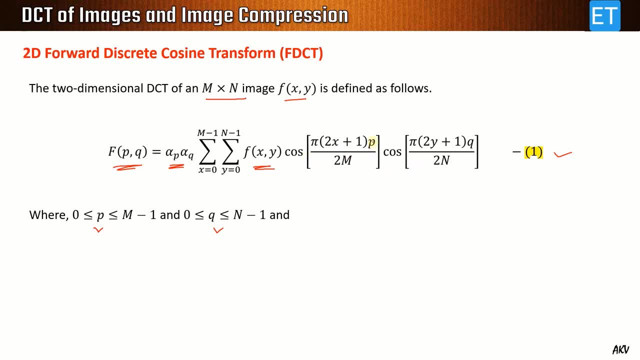 from 0 to n minus 1.. So how to compute this equation? First, we substitute the values of p and q. For example, I substitute, let's say, p equal to 0, q equal to 0. then I vary from, I vary x and y. 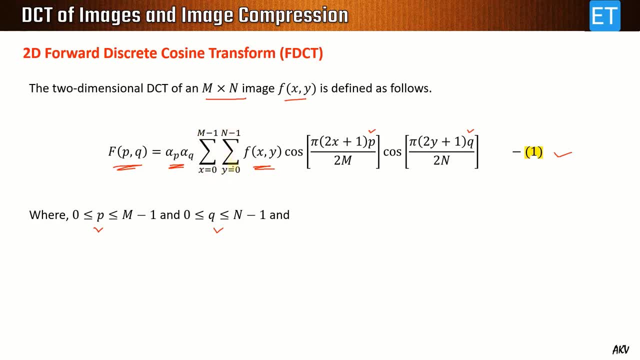 both from 0 to m minus 1 and 0 to n minus 1, and after that we change the p and q, for example p equal to 0 and q equal to 1, and then again varying x and y. So similarly, by covering all p and q, 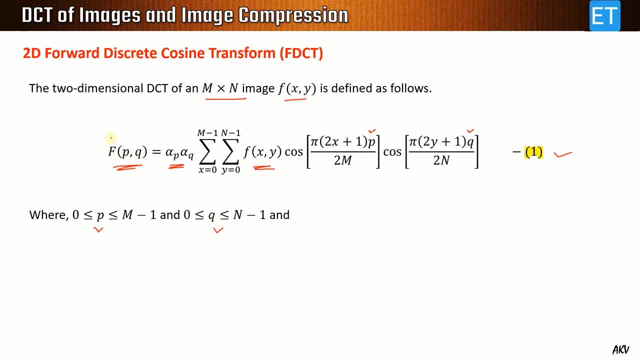 values in this range. you can compute this f, p, q matrix, which is carrying all the DCT coefficients, and these coefficients, alpha p and alpha q, are given by these equations: For p equal to 0 and q equal to 0, they are simply calculated by 1 upon square root m and 1 upon 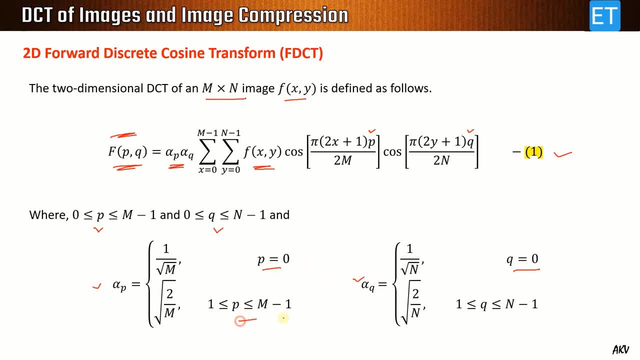 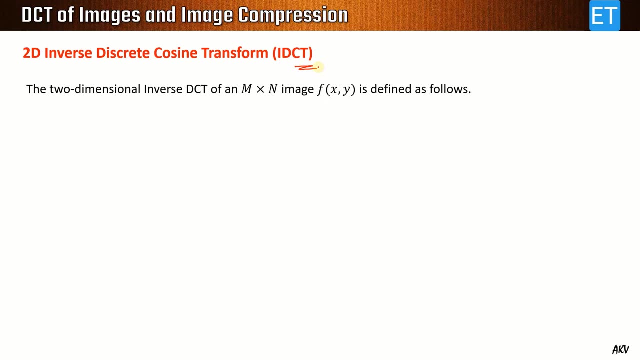 square root n and other than p equal to 0 and q equal to 0 values. they are simply equivalent to square root 2 upon m and square root 2 upon n. Now let us see how we can compute the inverse transform IDCT. So for an image fxy of size m by n, the inverse transform can be achieved. 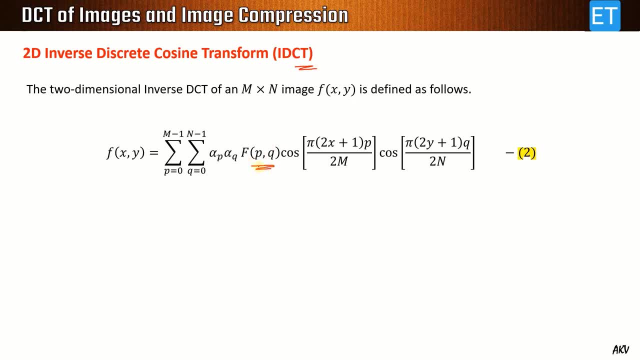 by the inverse transform of the inverse transform. So for an image fxy of size m by n, the inverse transform can be achieved by this equation. So this was your matrix, which is computed by the equation 1.. I mean it is carrying all the discrete cosine transform coefficients f, p, q, and now we are. 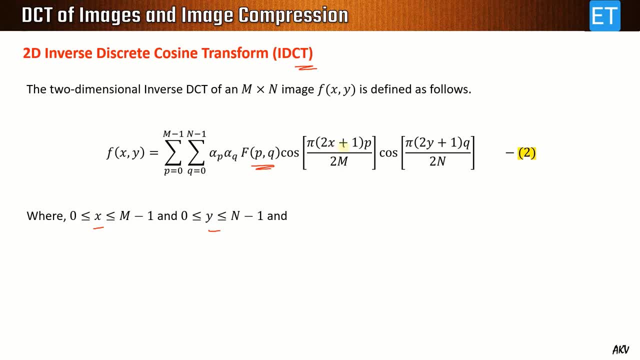 varying x and y. So here we are substituting x and y first, So substituting, let us say, x equal to 0 and y equal to 0, then varying the loop for p and q. Similarly we will write: x equal to 0, y equal to 1. 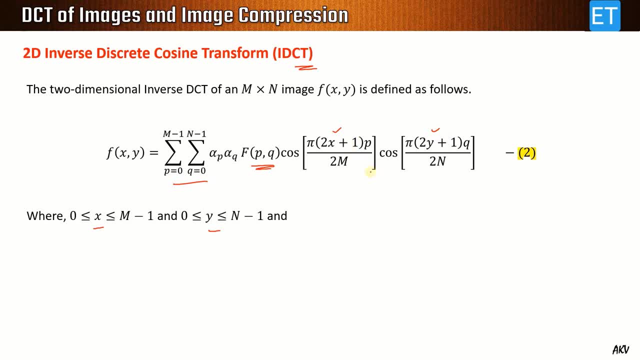 then varying these two loops again. So here you have to implement four for loops again. So the procedure is similar, similar as we have applied for fdct. Okay, and the equations for alpha p and alpha q remain same when you compared with that equation 1.. So this part is same. So if you 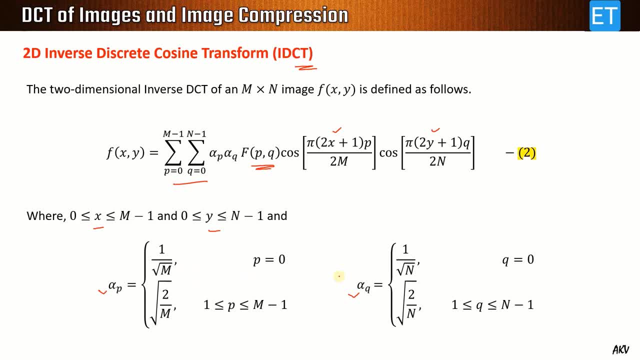 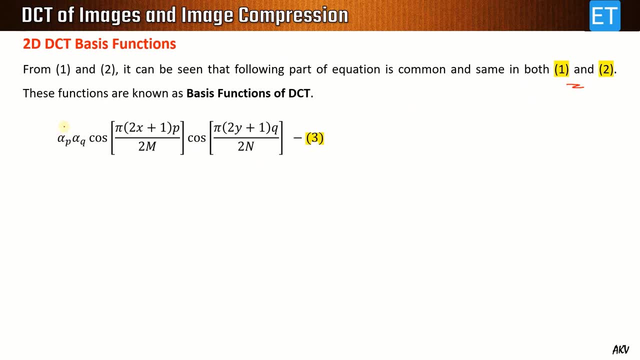 compare equation 1 and equation 2, you will see that this part is the same as the equation 2.. This is common between these two equations 1 and 2.. So that is alpha p, alpha q, cos, pi 2x plus 1 p. 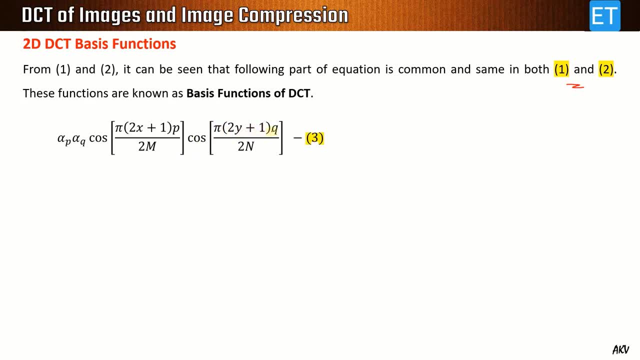 upon 2m and then cos pi, 2y plus 1, q upon 2n. So this part actually is known as the basis functions of dct. So here, if I can vary p, q and x and y, all four variables, I can generate the basis functions. 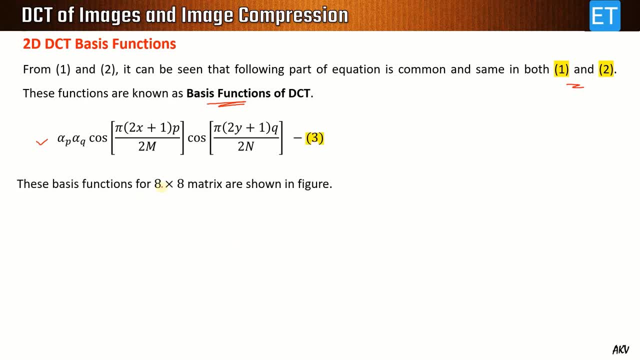 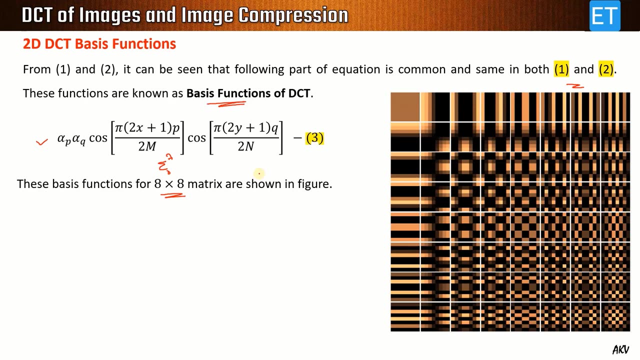 for two-dimensional dct. So for example, let us say my image size is 8 by 8. So suppose my all the four loops are varying from 0 to 7. I mean 8 times. then I can generate this type of basis functions. 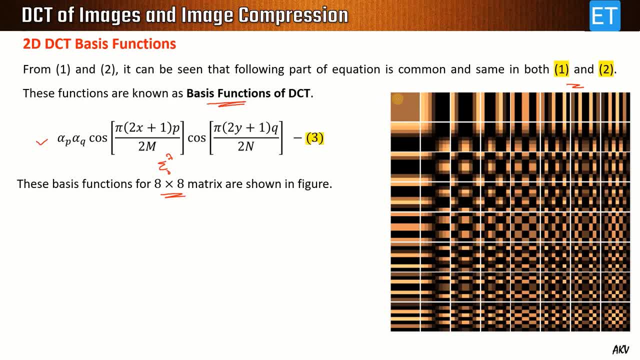 Okay, so this is for p equal to 0, q equal to 0. Okay, and this is p equal to 0, q equal to 1, and so on. So here you can see that the horizontal frequencies are increasing from left to right. So 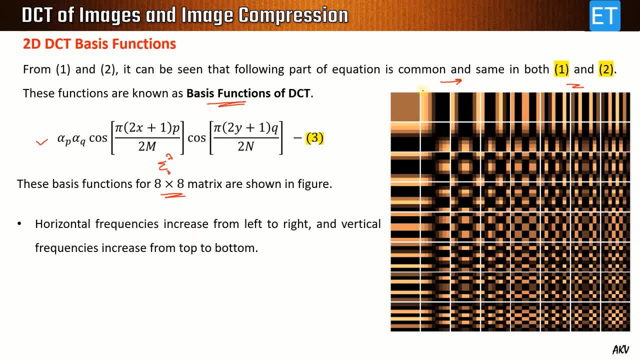 if you go from left to right, you can see that horizontal frequencies are increasing, And if you go from top to bottom, you can see that the vertical frequencies are increasing. So this is known as the dc basis function And it can be used to compute the first dct coefficient, that is. 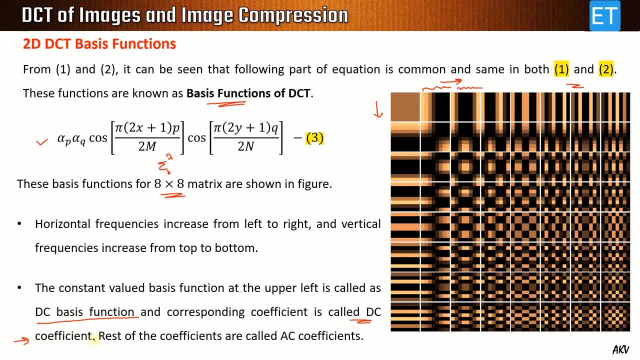 also known as the dc coefficient of dct, While other coefficients are known as ac coefficients, because in the first coefficient we get a constant value. So constant value is representing actually the zero frequency. that's why it is known as the dc- content of the image, While all other 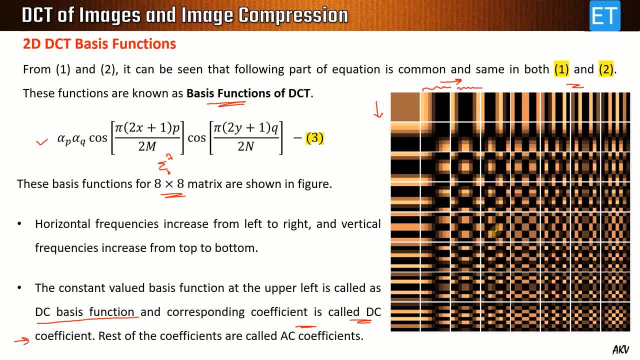 coefficients are carrying the varying values. that's why they are known as ac coefficients of dct. So actually, what is the need of calculating the basis function? Actually, for a particular size, let's say 8 by 8, we can compute these basis functions and we can store them into an array. 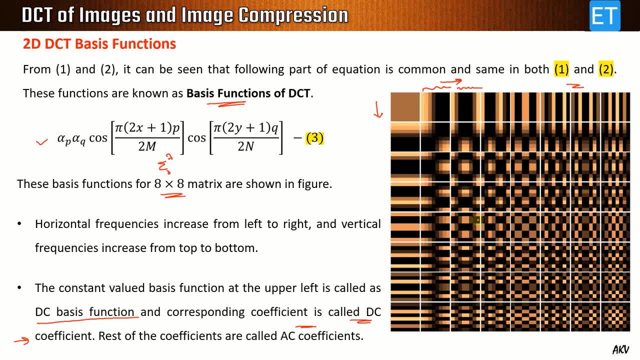 And later they can be utilized to compute the dct of a particular image segment of 8 by 8 size. Okay, so this is the basic function of the dct function, So we can compute the dct function of a particular image segment of 8 by 8 size. okay, so this? 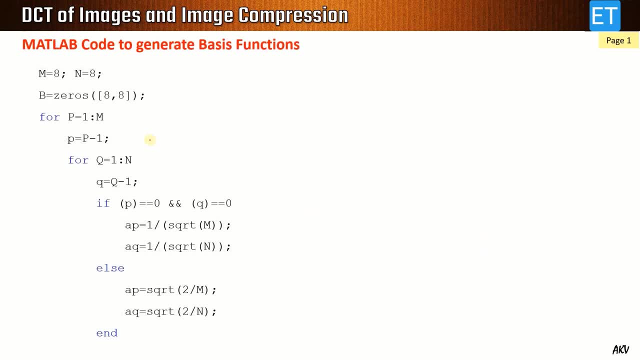 is the MATLAB code to generate these basis functions. So here we are, taking m equal to 8, n equal to 8 means I'm taking a small image segment of 8 by 8. And then just initializing this matrix and, as you can see, you have four for loops. 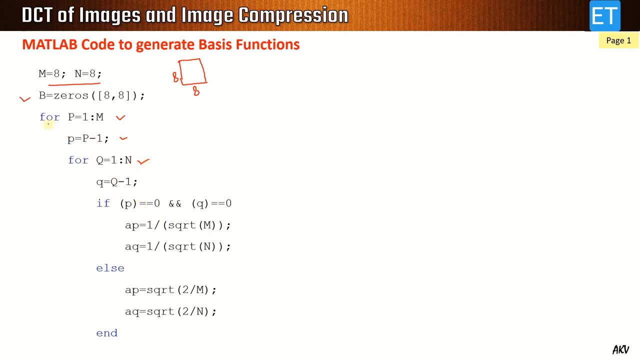 Okay, so one where p is varying from 1 to m. Actually, MATLAB index is starting from 1.. So to compute sigma, let's say p equal to 0 to 7, I'm just subtracting 1.. So small p equal to capital P minus 1.. This it is for. 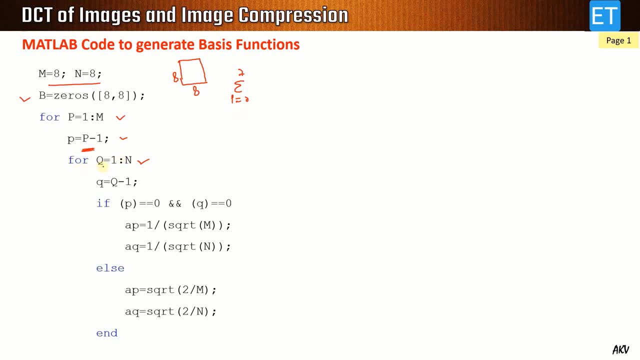 adjusting the indices. So, and similarly, the q is varying from 1 to n, If you remember this equation, where p is varying from 0 to m minus 1. And q is varying from 0 to n minus 1. okay, And here, with these conditions, I am. 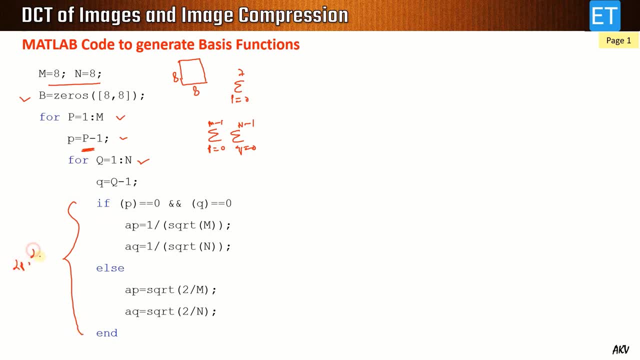 actually calculating the two coefficients alpha p and alpha q. If both p and q are 0, then alpha p and alpha q. both are square root m and 1 upon square root m, If you remember from the previous equations. otherwise they are simply square root 2 upon m or square root 2 upon m. 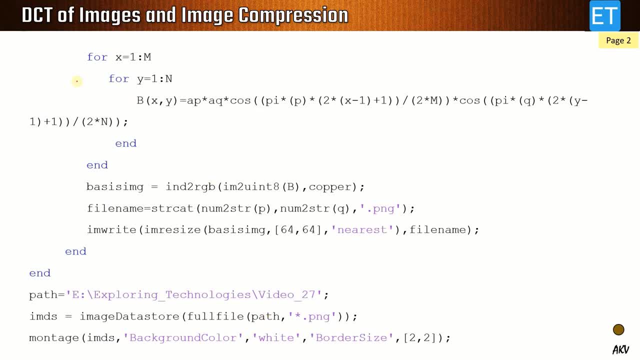 Okay, and in the next part these are two for loops, for x and y, So there are total four for loops. So here we are computing that equation. So that means this is your alpha p into alpha q, into cos, pi, p, 2, x plus 1.. Again, x is modified as x minus 1. 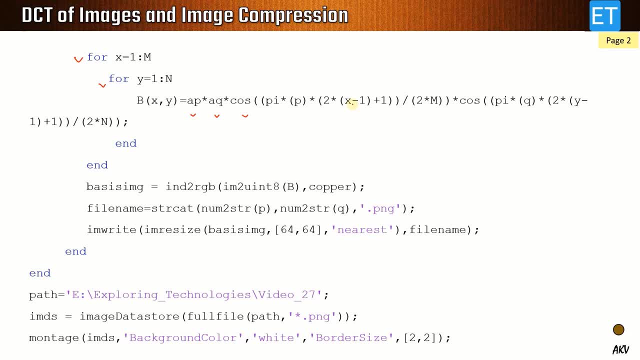 because MATLAB index is starting from 1 instead of 0.. Okay, And this is your cos: pi q, 2 y plus 1 upon 2n, So that equation is written And here the computation is done. But here actually I am converting all those computed. 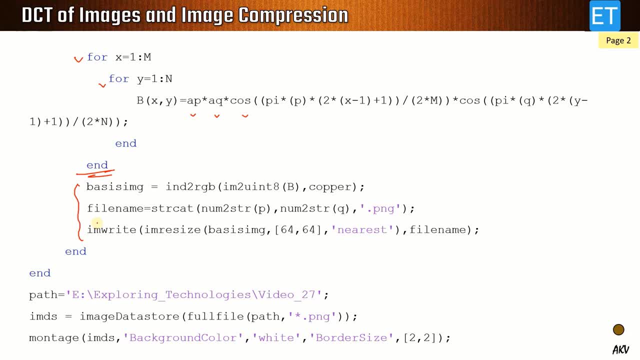 matrices as image. So later I will display all those images in combined format, as I have shown you. So here you can see that computed image is first converted into unsigned integer 8 and then converted into the RGB with the color map of copper. You can use any of your color map, for example the pink jet, etc. And I'm 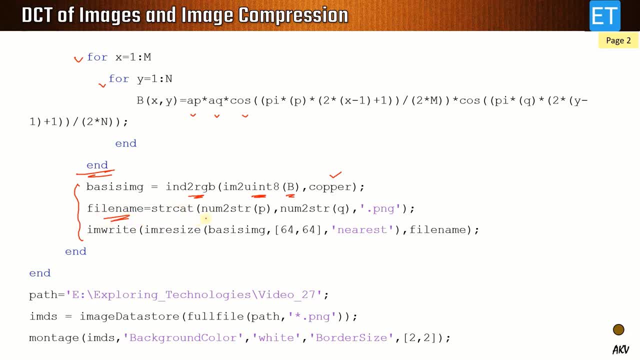 defining the file name by which I will save this image. So I'm saving the image with the name p and q. Okay, So you will get the images like 0, 0 dot p and g, or 0, 0 dot p and g, when both p and q are 0. And the next will be the 0: 1 dot p and g. and. 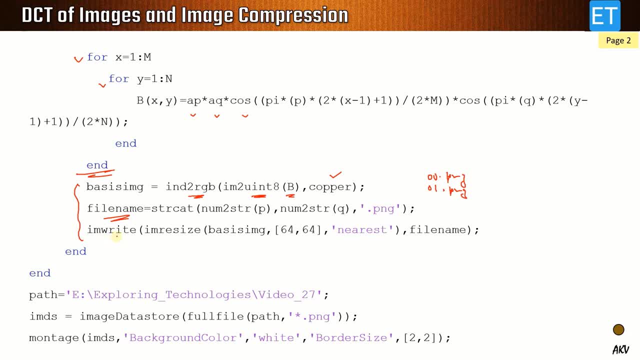 so on. And then I am writing all those images in 64 by 64.. Actually the original image size is 8 by 8. So it is very small size to display, So I am just enlarging them so that you can clearly visualize their structure. 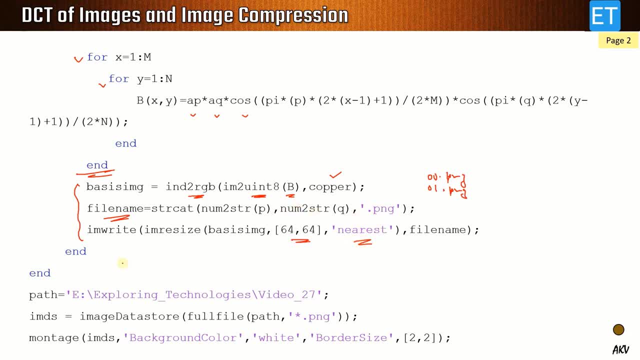 Okay, Okay, So I am displaying all those 64 images calculated in a montage by the montage command. So montage command actually is reading all the images which have written in the current directory You can see e exploring technology, slash video 27.. So, using image data store, I am reading: 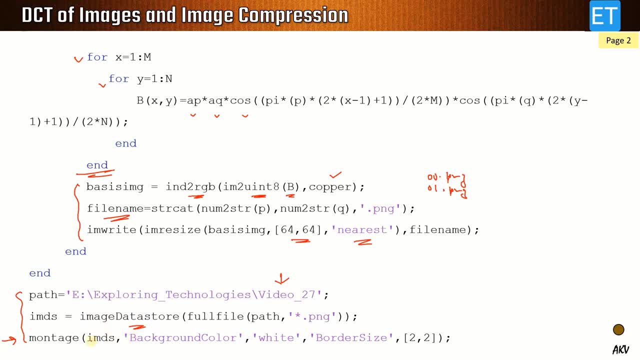 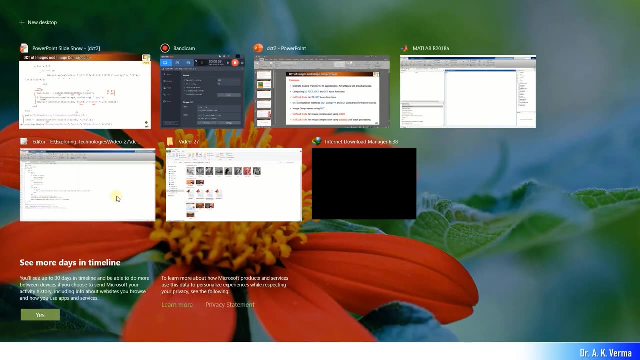 all the images. Okay, So all the images are now displayed in that 8 by 8 format. Okay, So let me run this program and I can show you that how these basis functions are calculated. So let me go to the editor. 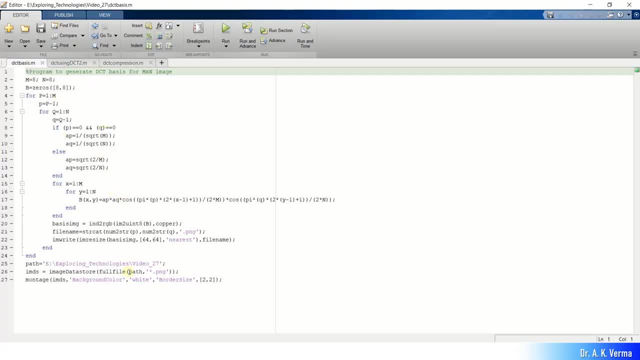 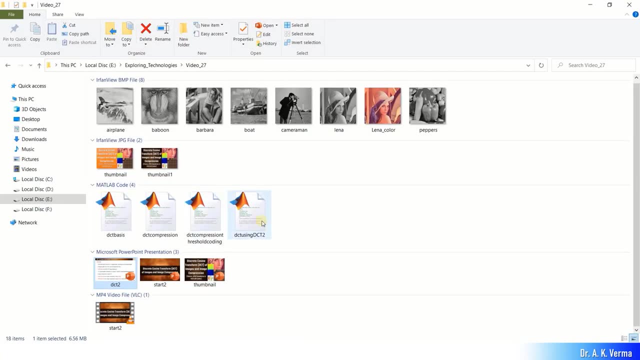 So MATLAB editor is here and this program is already written. So I am just pressing this run button And let me show you my current directory also. So this is my current directory. So no image you can see. You can see related to those basis functions. So after execution of that function you must 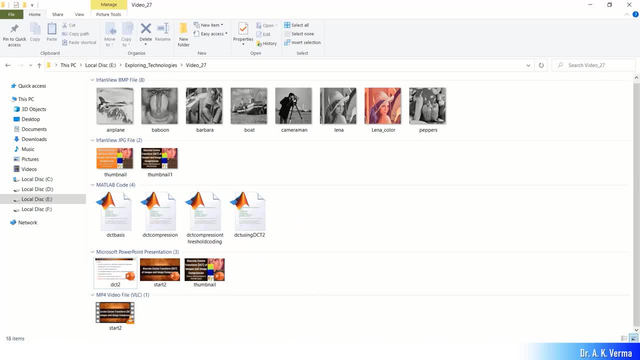 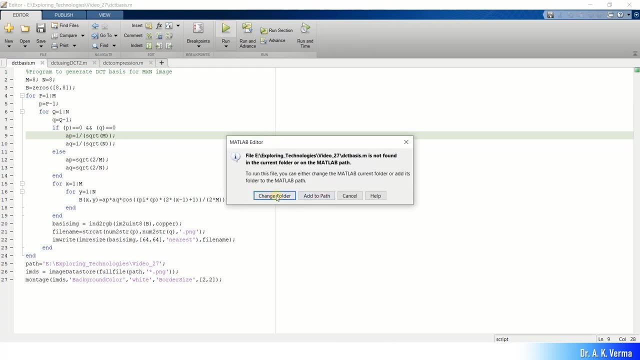 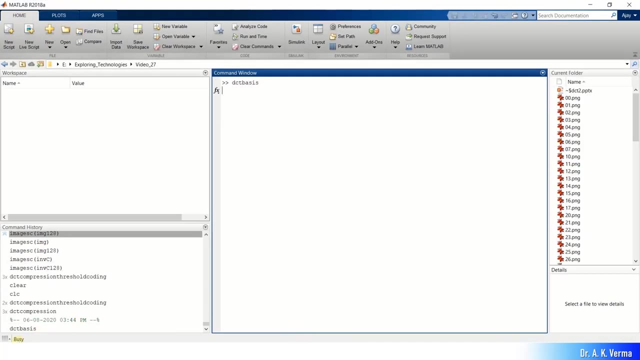 be able to see all those 64 images here. So I am running this program. Okay, Pressing this button, Change folder And this program is running. You can see MATLAB is busy. Okay, You can see. this is the output which I am. 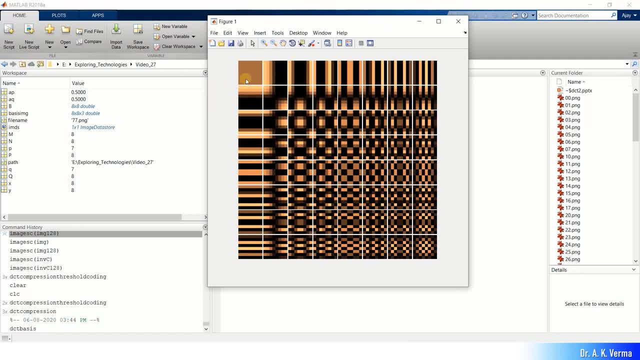 running. So here all 64 images of size 8 by 8. you can see This is your first coefficient, which is constant. And then, here you can see, the horizontal frequency is increasing Here, vertical frequency is increasing like that. So these basis functions can be utilized to. 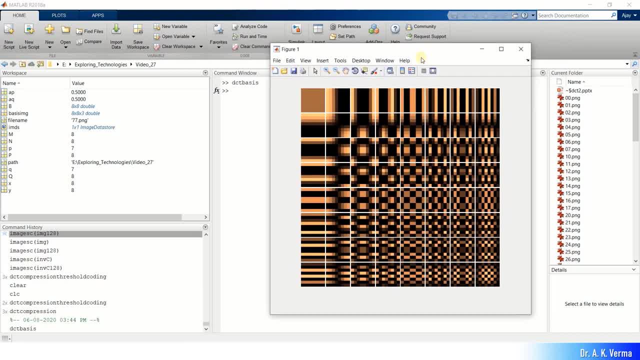 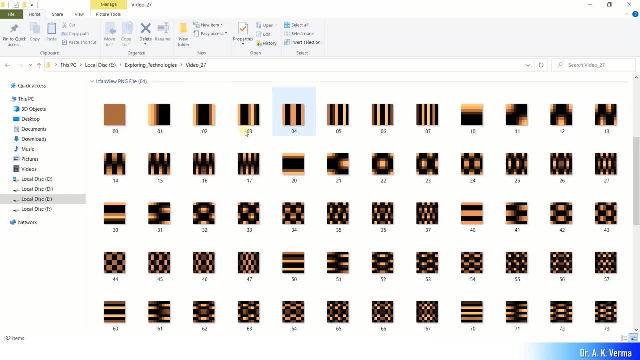 compute the DCD coefficients. Okay, And let me see my current directory. And yes, in the current directory you can see all these images. Okay, So I am running this program. Okay, So I am running this program. Okay, You can. 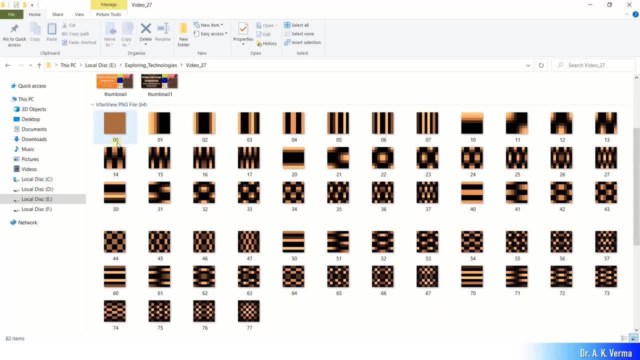 see, 64 images are saved. So first image is 00.. I am in the P equal to 0, Q equal to 0.. Then P equal to 0, Q equal to 1,, 01,, 02,, 03, like this up to the 77.png. So all 64 images. 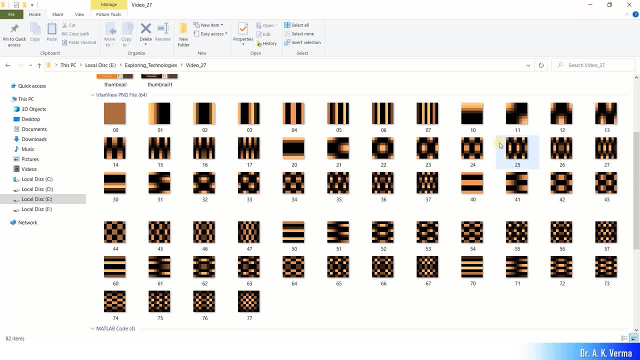 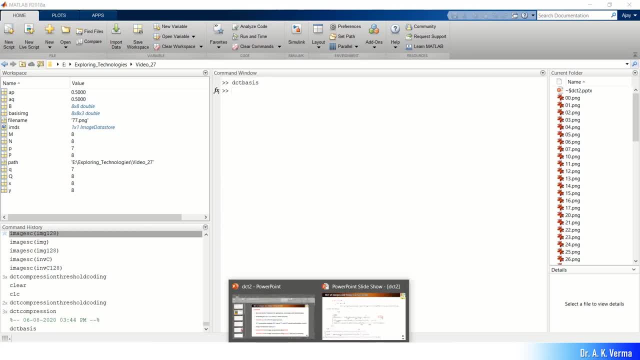 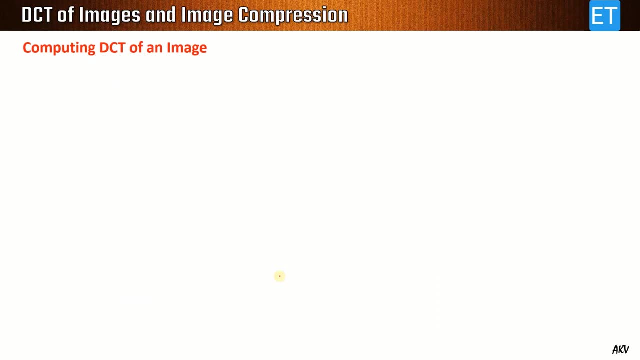 are here. You can change the- actually the color map to represent these into the different color styles. Okay, So now let me come back to my presentation. Okay, So now let us see how we can compute the DCD of an image. Actually, we can compute with. 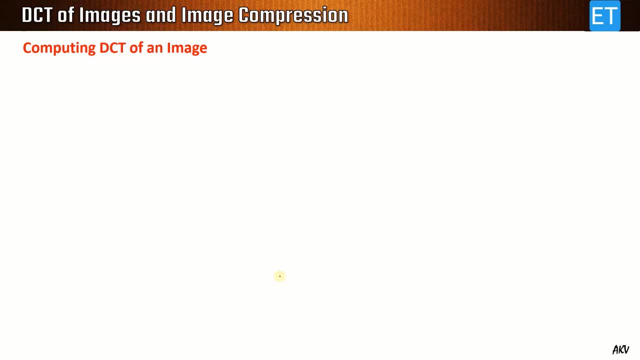 help of these basis functions also. But this will is not a flexible approach, because once the DCD basis functions are computed, they are fixed for a particular image segment. I mean, if you compute this for 8 by 8, then you can apply the DCD on only on the 8 by. 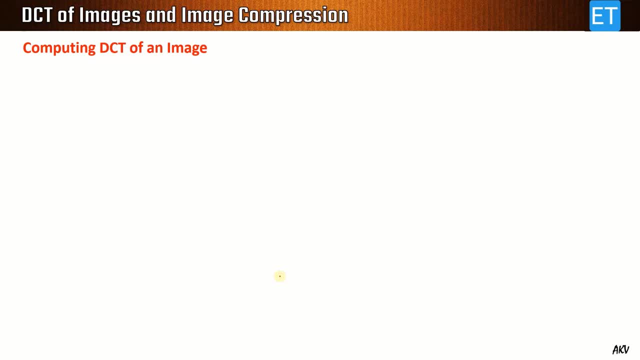 8. Okay, So that is not a good approach. Actually, we have two different approaches, Okay. So the one is the transformation matrix approach and the second is the FFT based approach. So let us see first one, the transformation matrix approach. So this method is suitable. 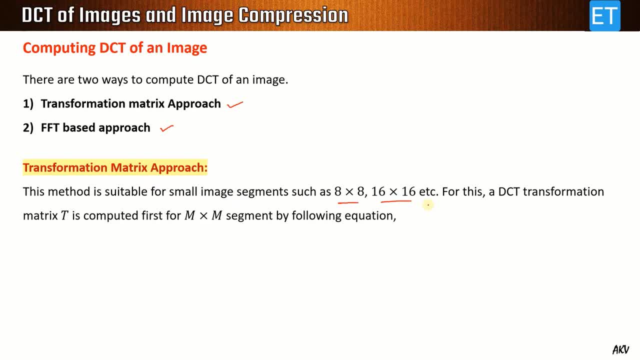 for small image segments such as 8 by 8,, 16 by 16, etcetera. For this DCD transformation matrix T is computed first for an M by M image segment by following equation: So this is the equation by which you can compute a transformation matrix for a M by M image segment. Okay, 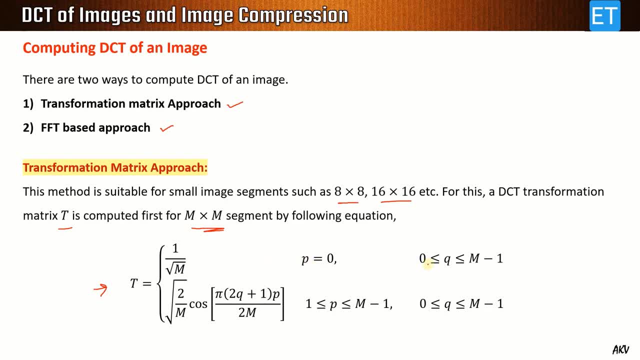 So here you can see that for P equal to 0 and Q equal to 0, there is 1 upon square root M, or for Q from 0 to M minus 1, it remains the same value. So that means the first row will have the same value, 1 upon square root M, for all columns. After that it will change. 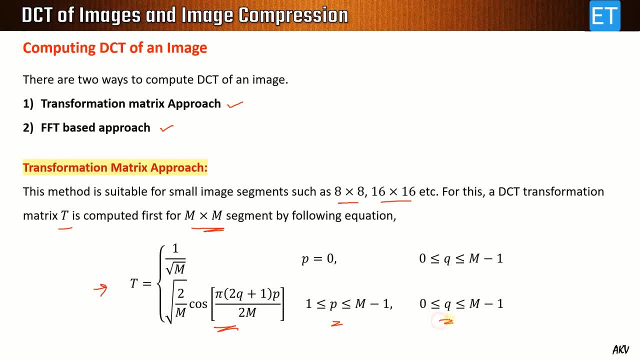 to this value, depending on the value of the image segment. So the first row will have the same value, 1 upon square root M, for all columns. After that it will change to this value, depending on the value of P and Q. Once this transformation matrix is computed, you. 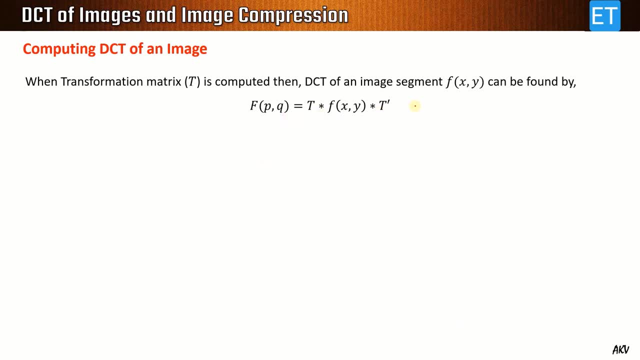 can find the DCD coefficients of that image segment by this equation. So here you can see that this is your image segment. So this is your image matrix, then multiplied with this T matrix, then multiplies with this T transfers matrix. So if you do this simple, 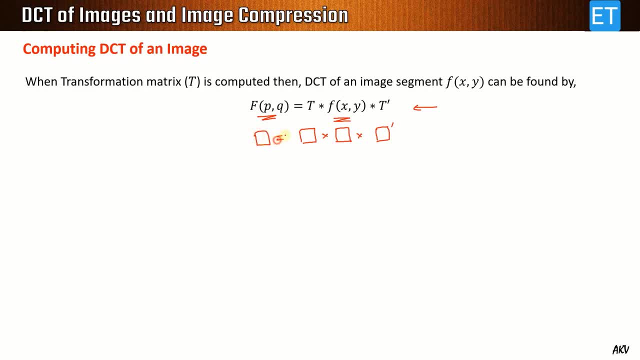 operation, you get the DCD coefficients matrix. Okay. And similarly you can find the inverse also, Since T actually it's a real orthonormal matrix, So its inverse is equivalent to its transpose. So therefore inverse DCD can be found by this equation, So you can recover your image effects by by this inverse operation. 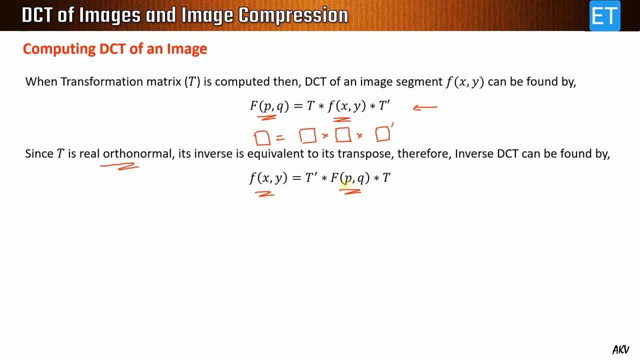 So this is FPQ, is your DCD coefficient matrix, and then same matrix, transformation matrix, is put here, T, And then you have to find T functions. So this is the inverse and we have R, W as required. So that means if we think about this equation we can see that it is. 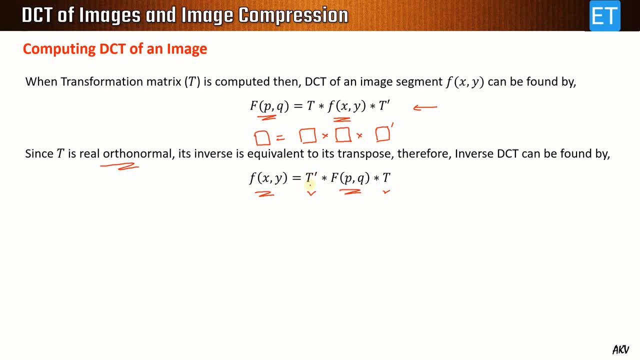 going to be the same thing we have never thought about. So it is going to be similar to the t dash, that means the transpose. so by this operation you can get your image segment fxy back. so in matlab dct transformation matrix t can be computed by executing this function: dct mtx. 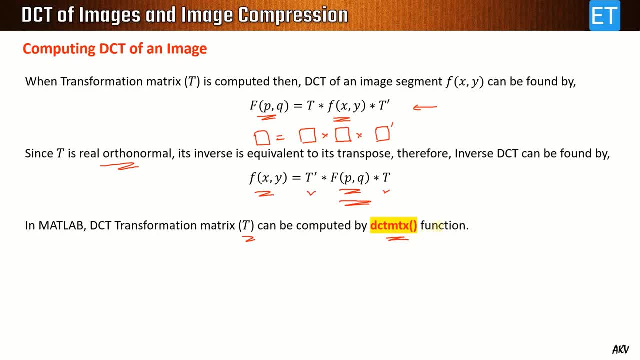 so if you execute this function, dct mtx, you can generate any size transformation matrix. and the second approach is based on fft. so this approach utilizes the fft structure for speedy computation of dct, so therefore it is suitable for large input images and in matlab it is achieved by executing this dct2 function. so if you go to find the dct of small image segments, 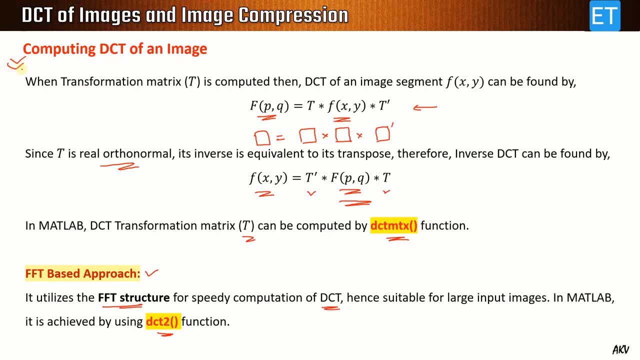 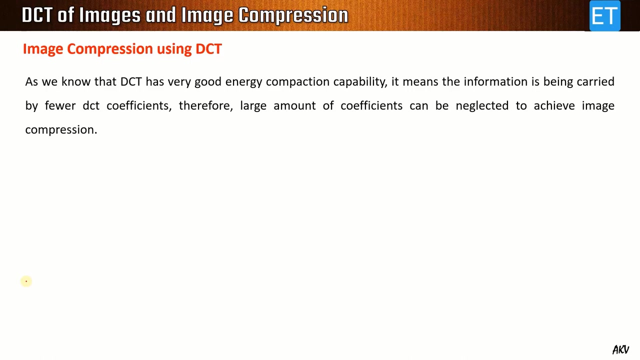 you must prefer the first one approach and if you want to find the dct of a large image, then you can go to this approach, fft based approach. okay, i will show you both the approaches by writing matlab codes, how they can be used for the image compression. now let us see the image compression using dct, how we can achieve actually image compression. 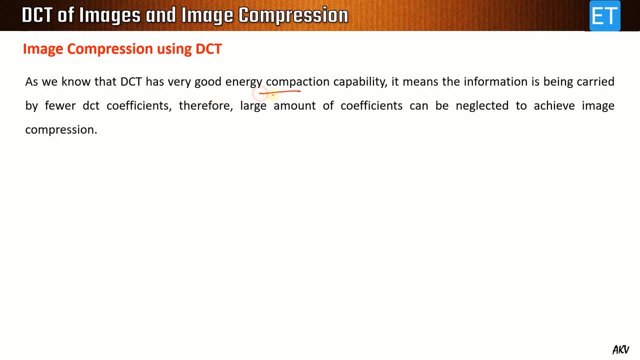 so as we know that dct has very good energy compaction capability, so it means the interaction between the image compression and the dct is very good. information is being carried by fewer dct coefficients, so therefore large amount of coefficients can be neglected to achieve the image compression. so that is the fundamental. 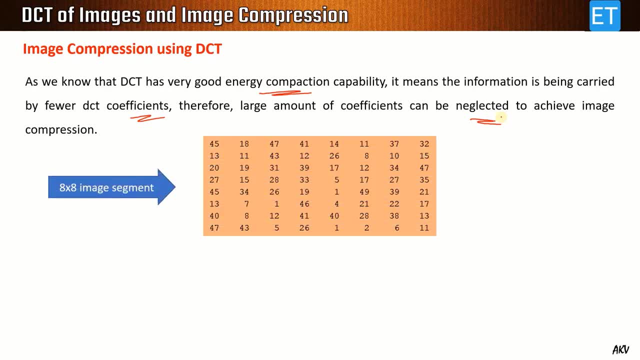 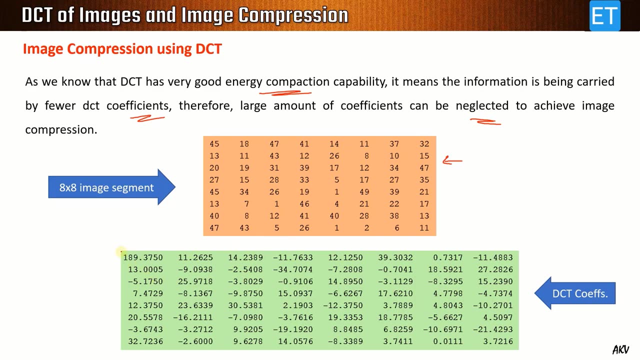 behind the compression. so here you can see one example. this is my 8 by 8 image segment. so you can consider this is your 8 by 8 image and if you take the dct of it, you can see these dct coefficients. so you can see this first one, which is: 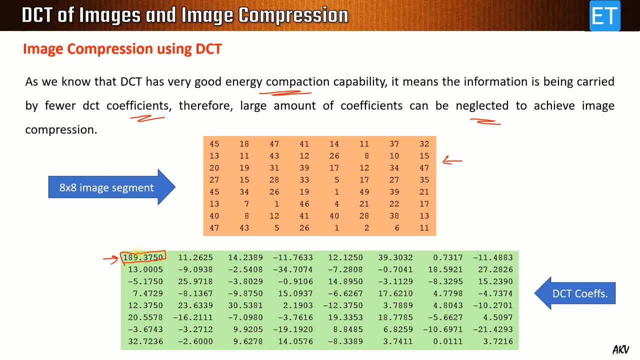 known as your dc component, which is the largest one in the dct coefficients and and just compare the other coefficients values, you can see they are very small in size. for example, 0.011 3.7 minus 4: 4 point point seven, three point seven. seven point two. point nine: you can see very small. 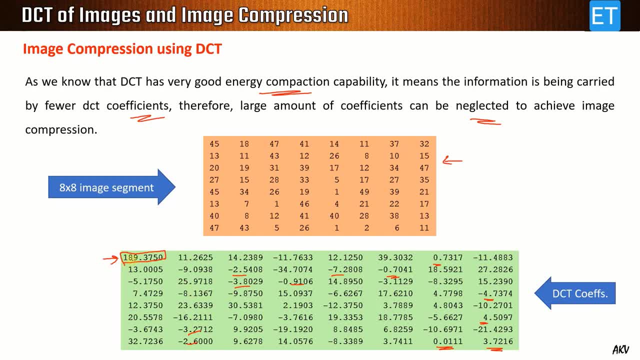 coefficients, uh, okay, uh, as computer. compared to this first one, even some larger coefficients are also there, like 11, 13, 12, 20, 35, 23, etc. so you can see that you can achieve the image compression by simply making these small coefficients uh to the zeros. that means this is known as the quantization. 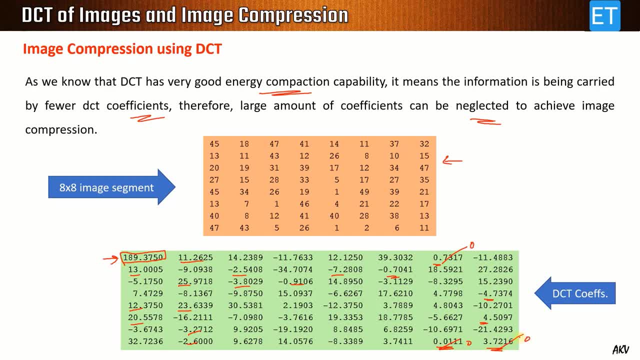 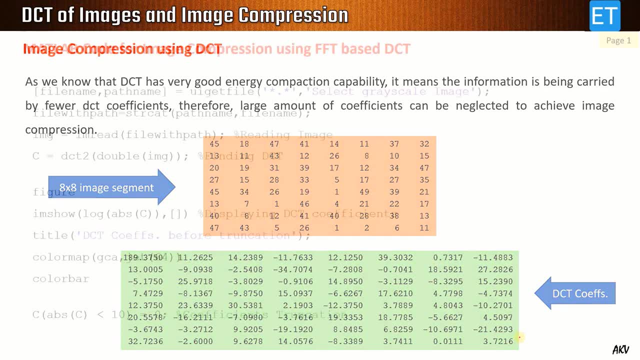 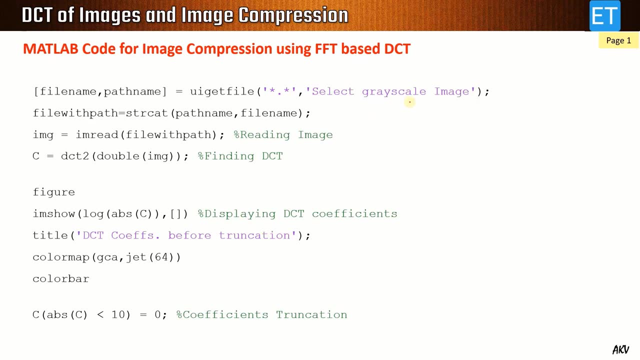 process, so you can simply make them zero. this is how you can achieve uh, the image compression, by making these small coefficients zero. so now let us go to the matlab port for image compression using the fft based approach. okay, as i have explained you, that fft based approach uh is achieved by executing this matlab function. 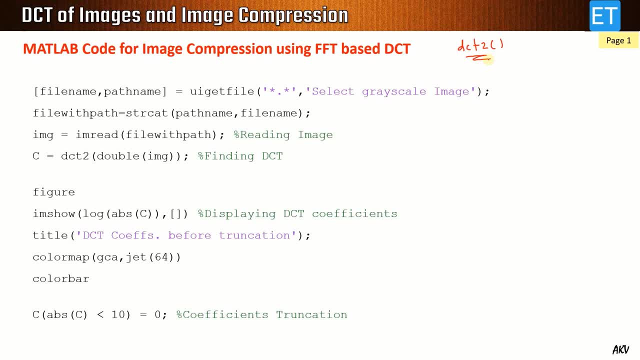 that is the dct2. so i'm utilizing this matlab function dct2 here in this case. so when you execute uh- the first few lines, you can see uh. with the ui get file you will get a system dialog box where you can choose your grayscale image and then your image is read by this: im read and your. 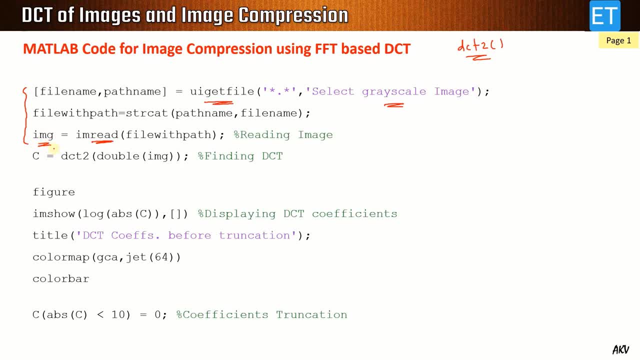 whole image information goes to img variable. then with this function dct2- you can see here i'm taking the discrete cosine transform of this image. so dct2, of this image, all the dcd coefficients will go to this matrix c. so here i am actually showing you the dcd coefficient matrix. 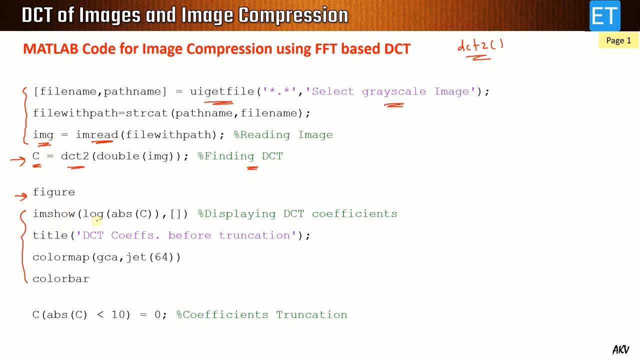 with this command, i am sure, just taking log to highlight the coefficients differences, if you, if you don't take log, you will get a black or dark image. otherwise you have to take log so that you can differentiate the magnitudes clearly. so taking the absolute values of c and then taking log, you can display these dct coefficients properly. 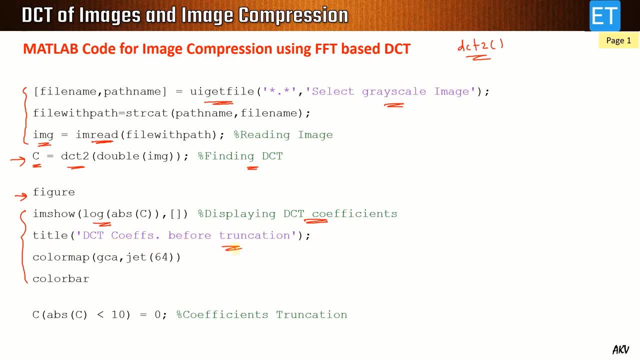 so with the title dcd coefficients. before truncation. i have not used any truncation here. they are just original dct coefficients and for representation i am using the color map of jet with a color bar. now i am doing the truncation process, so that is a coefficient. 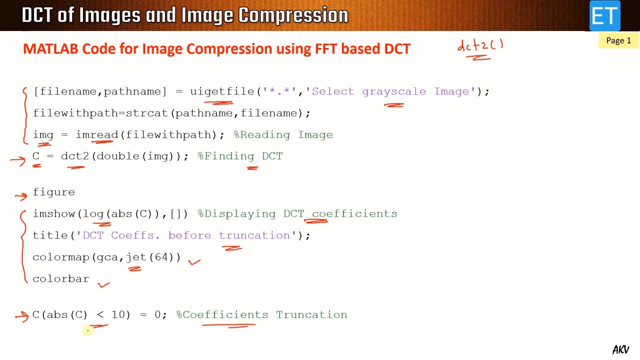 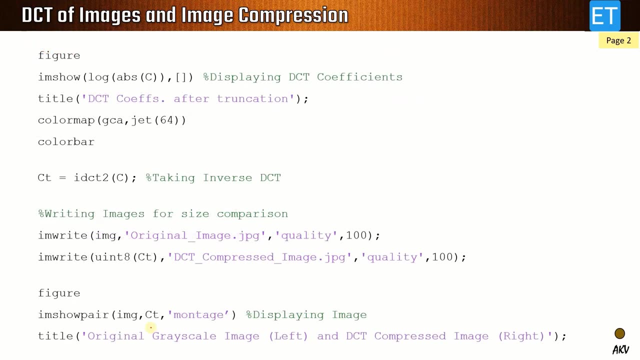 truncation. here you can see that all the coefficients of c which have the value less than 10. they are simply neglected and that means they are made to 0. so this coefficient truncation is done with this equation, and then now you can display the truncated dcd coefficients in another image. so for that i am taking the. 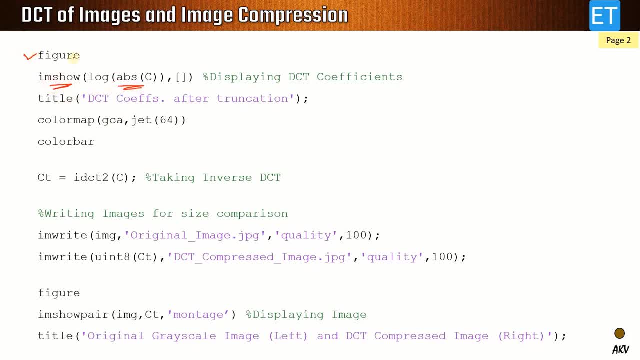 another image and i am showing all those truncated coefficients so you can have the comparison between the truncated before truncation and after truncation, so you can compare those dct coefficients. then i'm taking the inverse discrete cosine transform with idct2 function. so this is my actually. 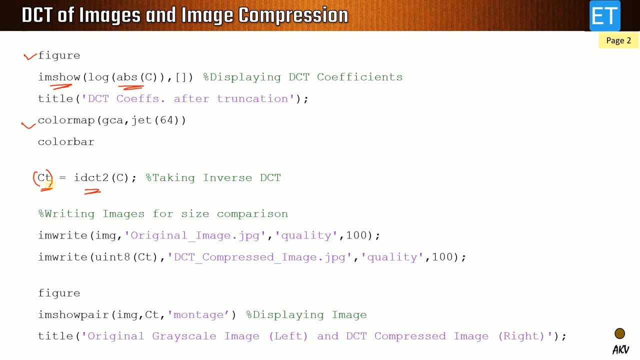 the recovered image, but it is in double data format so i have to convert that into a proper image format. so for that, i am just writing this image into the current directory in form of jpeg with the quality 100. so what i am doing? i am writing the original image, img, and i am writing. 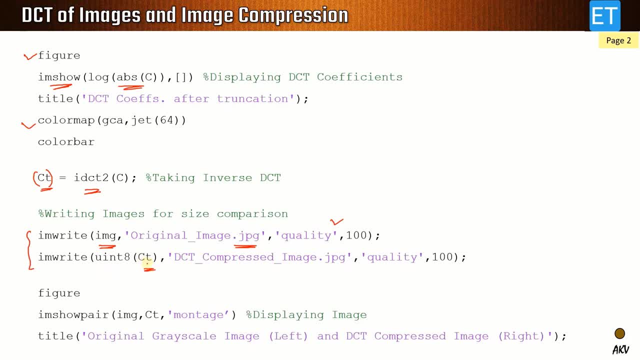 this reconstructed image, ct with the same quality, index 100. okay, so both are in jpeg format so you can compare the size of these two images. i mean the original image and then reconstructed image after the dcd coefficient truncation. so, and here i have shown both the images side by side. 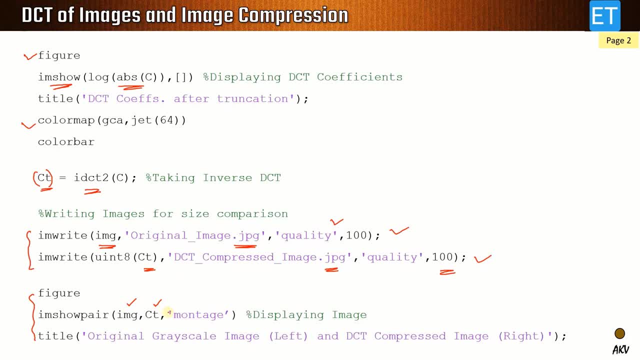 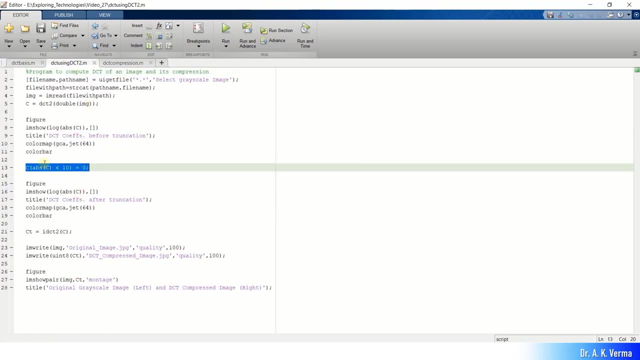 i mean your original image and the reconstructed image, so you can have the comparison of the quality. so let me run this program in the matlab, so let me jump to the matlab editor and this program is written already. so here you can see the truncation is done with this equation. 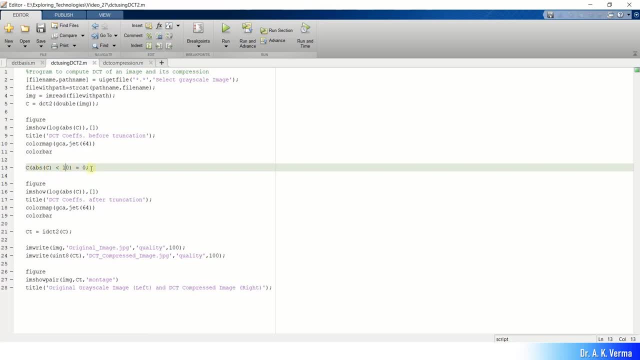 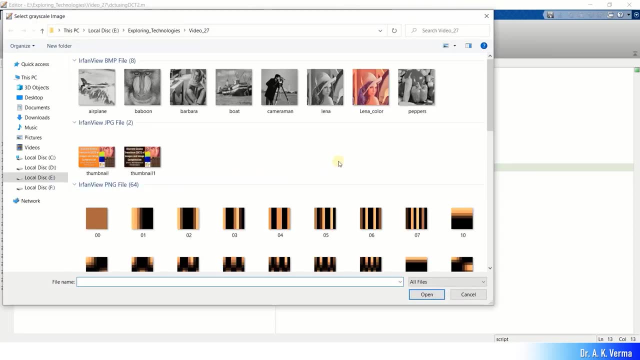 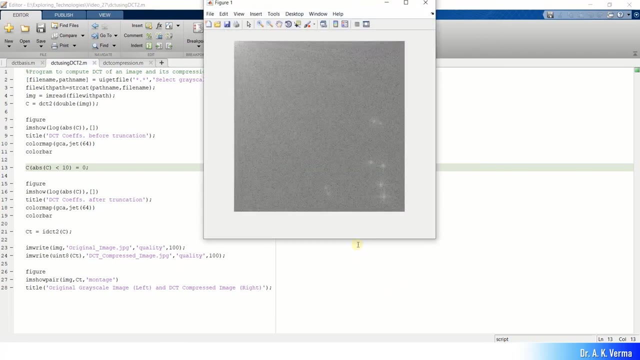 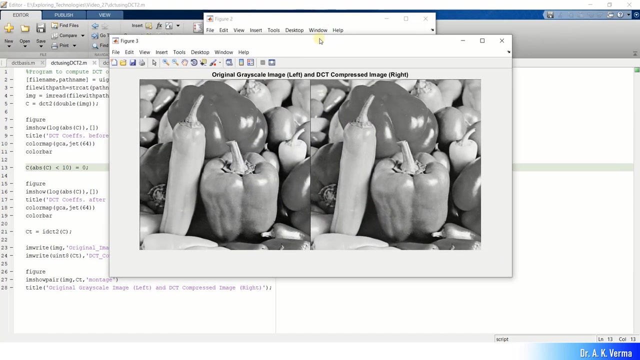 that means all the coefficients having values less than 10 will be made zero. so let me run this program and it asked me to choose the file, so i am taking this paper image and here you can see the various coefficients. yes, here you can see the two images side by side, so this one is your original image. 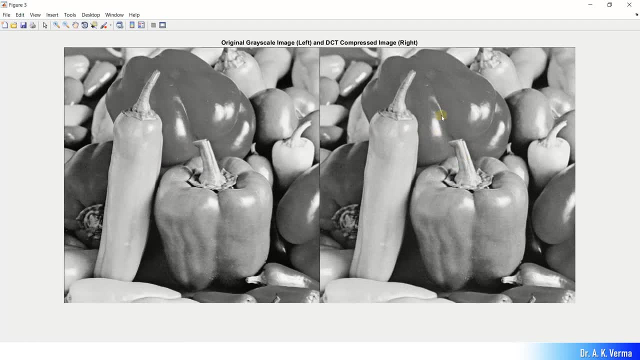 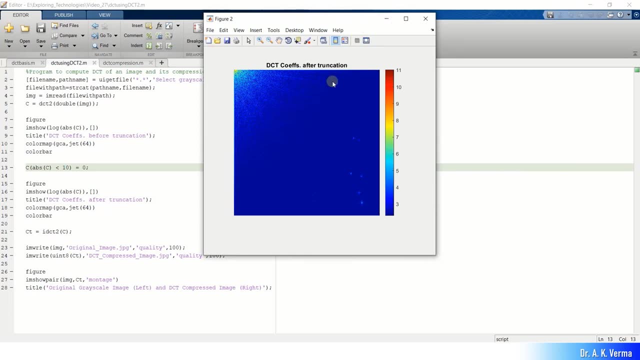 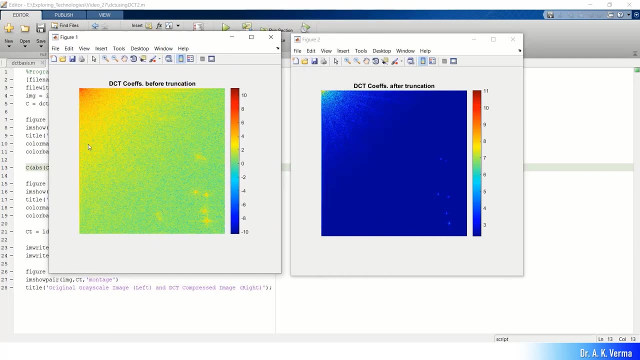 and this is your dct coefficient and this is your uncompressed image. okay, so quality wise there is no difference almost. and here you can compare, uh, the dct coefficients before truncation and after truncation. so dcd coefficients before truncation you can see that this matrix has the color towards the red and 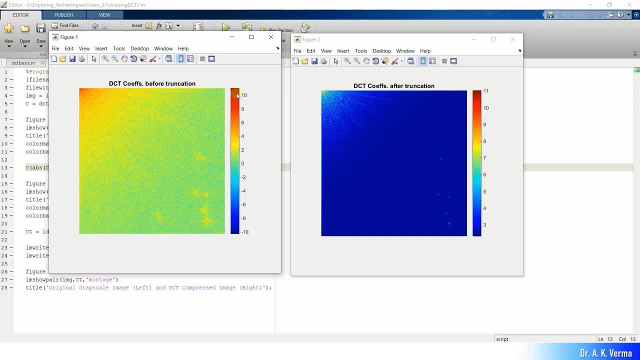 yellow it. so from the color bar you can see that these mat coefficients are at the higher side, so becomes blue. it means the coefficient values actually are now approaching to the lower side. okay so, because all coefficients above 10 are made to 0. so by this color information you can see that there is a reduction in the 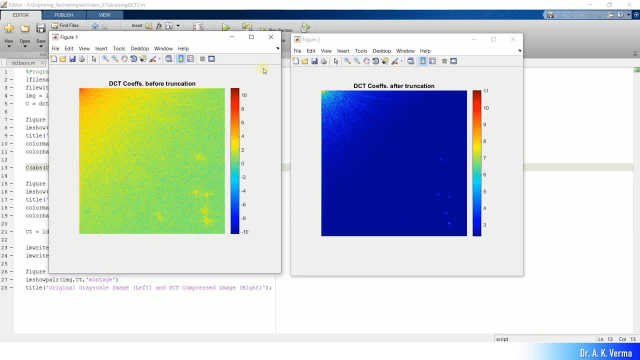 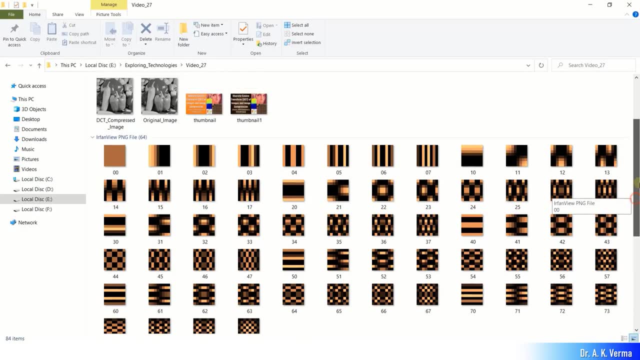 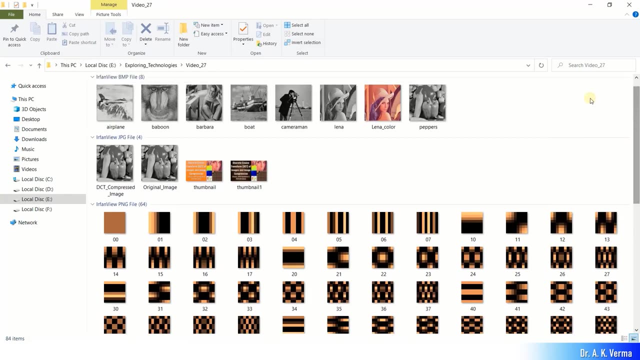 amplitude of these coefficients. so let me see actually the sizes of those images. so for that I have to go to my current directory and let me find those two files. I mean the original one and then compressed one. so here you can see that these two files, i mean the original file and then DCD compressed image. so 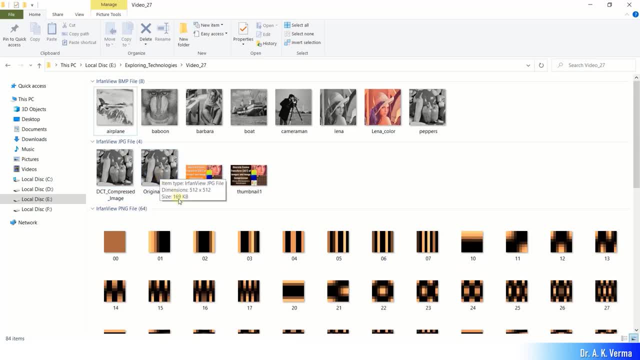 just place the cursor, its size is 169 kb, 169 kb. and now let me place the cursor on DCD compressed image. so here you can see that it says size is 159 kb. so there is slight reduction in the size. the original is 169 and after compression it 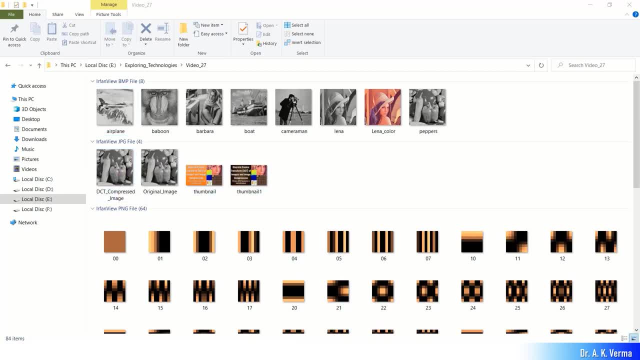 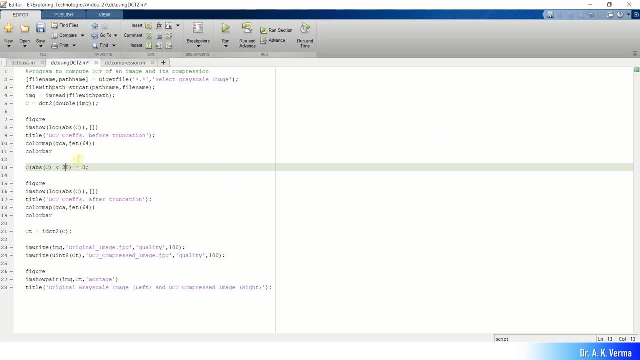 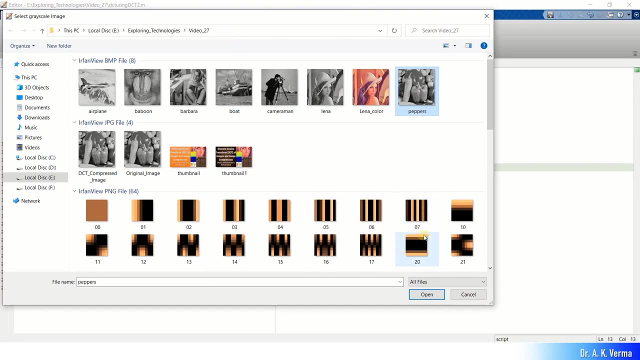 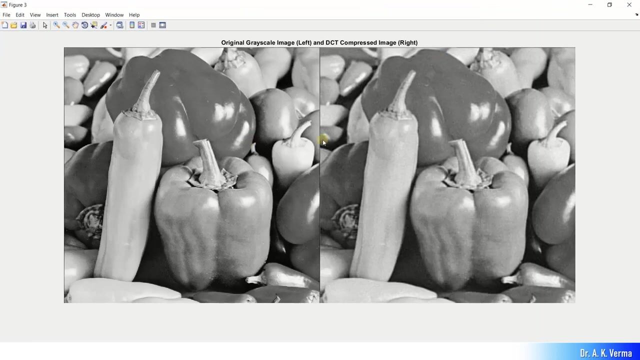 is 159. you can achieve more compression by neglecting the higher magnitude. so instead of 10 you just change it to 20 and let's see how much size reduction i can achieve. so simply run it and selecting the pepper open, and here i'm getting the original image and compressed image side by 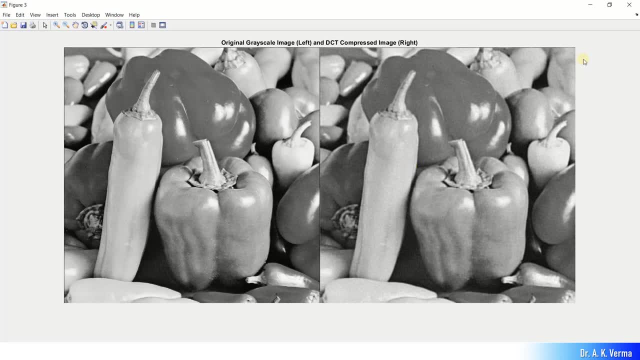 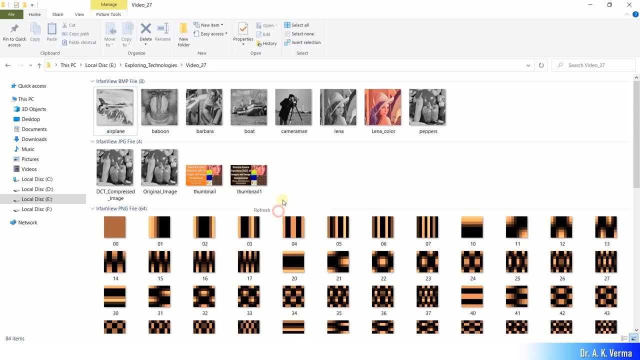 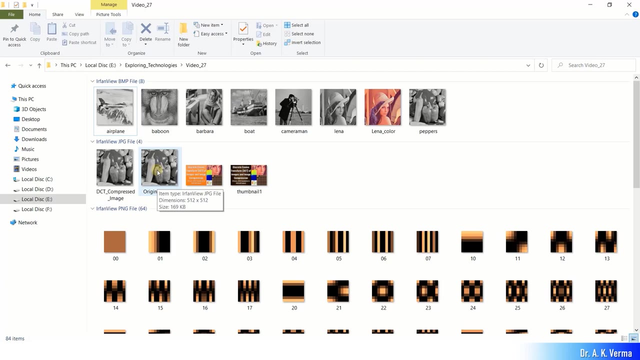 side. so again, there is not much uh change in the quality. and let me see the size comparison. so let me see what size i achieved. so just place the cursor and its size is obviously 169 because it is before compression and its size is 145. so initially it was 159, now it is 145, so i'm getting the reduction of 20 and more in this case. 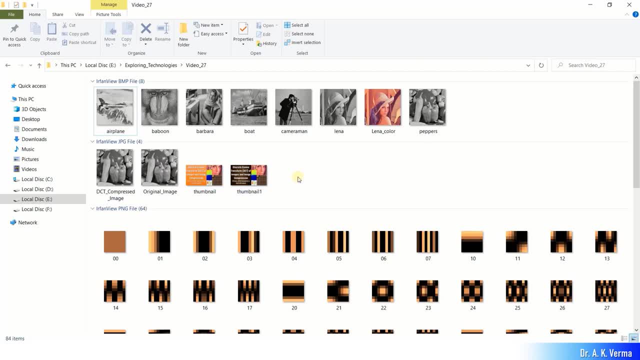 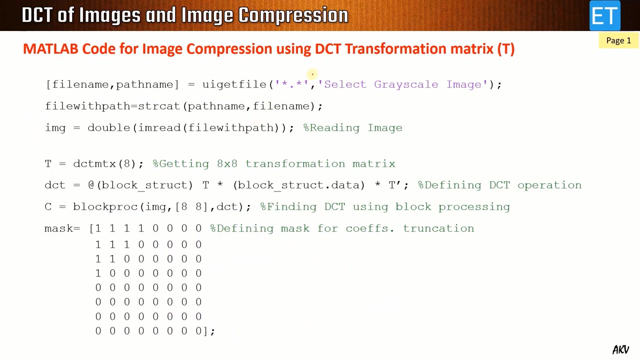 so if you truncate more dct coefficients, you will get more reduction, but at the same time the quality of the image will decrease. okay, so now let me come to my presentation back and i will show you the another example. now i will discuss the matlab code for image compression using the dct transformation. 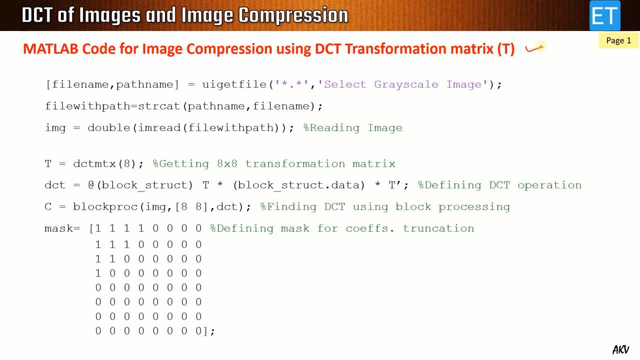 matrix. so this, this was another approach, as i discussed here, instead of using the dct2 matrix, which is which is based on fft approach, i'm using a transformation matrix approach which is suitable for a small image segment. so with these lines of code, you can see with the UI, get file again. you. 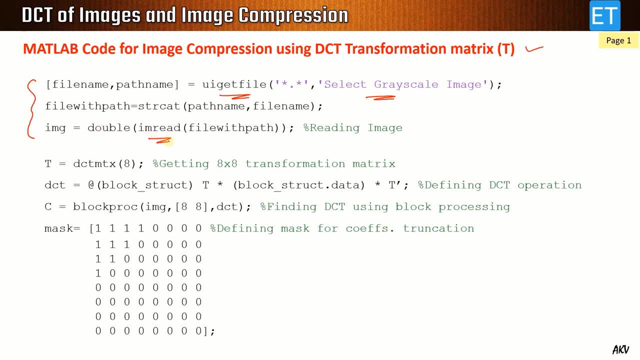 can select your image and the I am read is reading your image and putting all the information in IMG variable. now, with this equation, T equal to DCD, MTX it, I am getting the 8 by 8 transformation matrix. see my side. my image size is bigger it. 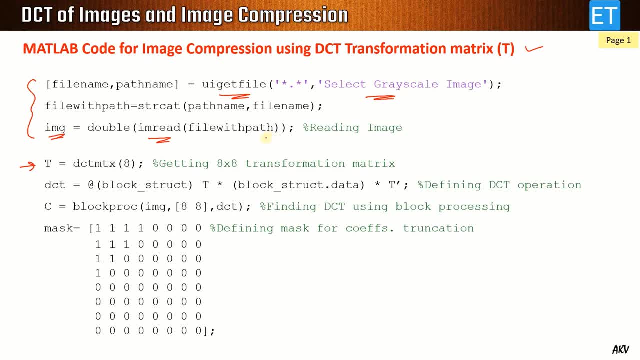 is not 8 by 8. my image size is 512 by 512, but I am taking the DCD MTX 8 by 8. okay, so what I will do now? I will divide my whole image, the bigger image, into the small image segments of 8 by 8. so I will now do the processing on this 8 by 8. 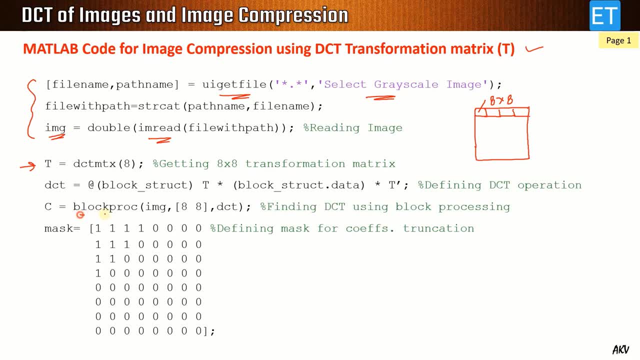 image segment. so that why I'm I'm using this block processing, which is a mat labs in built facility, to do this block wise image compression. so I will take one block of image at a time, then I will find its DCT and then I will neglect its. 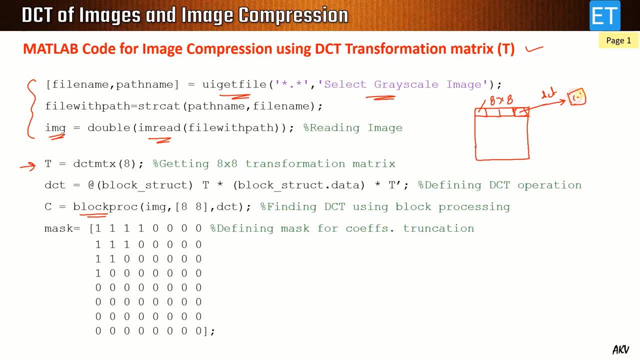 coefficients. I mean I will simply quantized it- coefficients. then I will take inverse DCT to get the image segment back and then I will combine all these 8 by 8 segments to make my image as a whole image. so here you can see that with this command I am just defining the DCT operation that will be applied on. 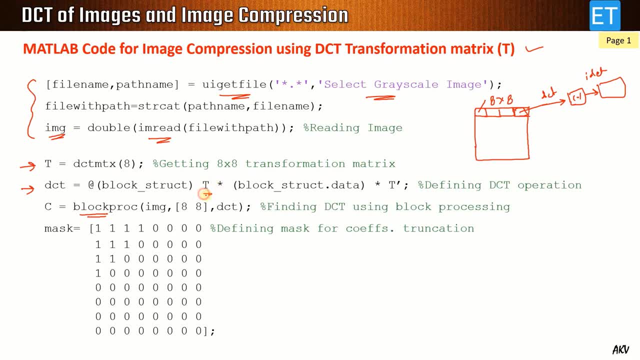 that image segment. so you can see that this transformation matrix T multiplied with the block structure dot data. it means that 8 by 8 block and then multiplied with T transpose. if you remember the DCT operation then it was a T matrix A, then multiplied with T transpose. so that is defined here now. 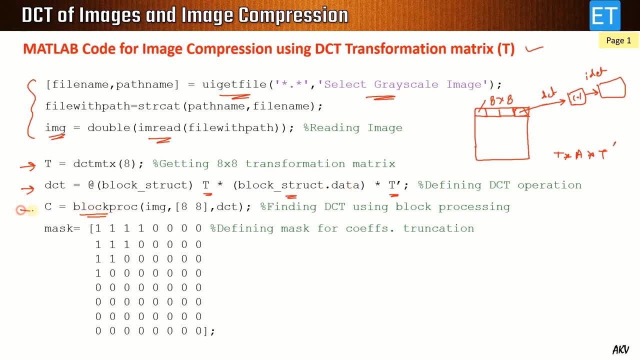 with the mat lab block processing function. I am computing the coefficients, DCT coefficients- of all 8 by 8 blocks found in an image. so here you can see that your image is passed. then here you are defining the block size and here you are defining the operation. this one, okay, this one here. so this block processing. 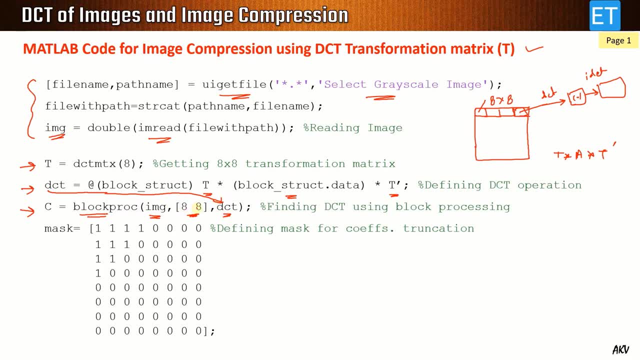 function. what it will do? it will take 8 by 8 blocks from image which you have passed and then it will do the operation dct. i mean this, this operation t a, t inverse, with each 8 by 8 block. so in this c you will get all the dct coefficients by this approach. now we are doing the coefficient. 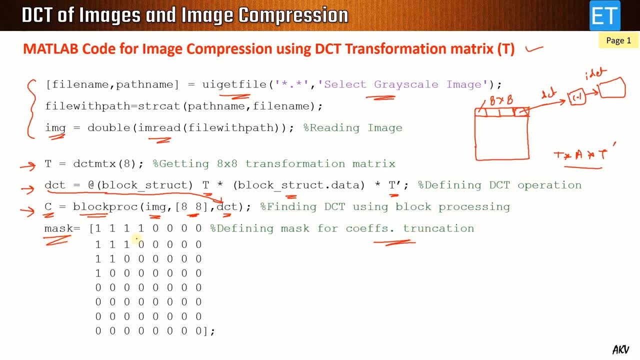 truncation. so i am applying the mask- it's a fixed mask and here you can see this mask- that all the coefficients are made zero except these coefficients. so these few diagonal coefficients, i mean from top left corner, are considered, because the first one you have to consider it in any way because it is your dc content which is the maximum coefficient. 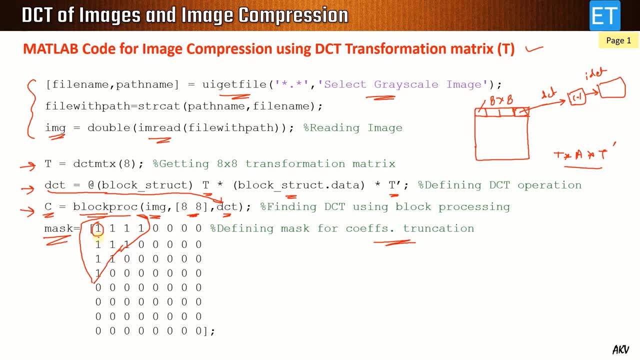 of your dc truncation and it is carrying all the basic information, and few high frequency components are selected. so this is how you can select your coefficients and how you can reject the remaining coefficients. so what i have to do, i have to simply multiply this mask to the coefficients, okay, 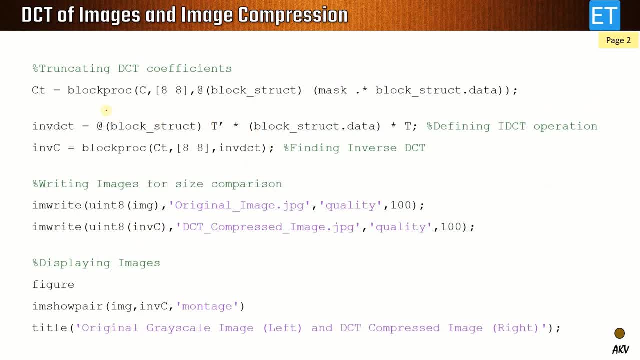 so again i have to do the block processing. so here you can see the in the truncation dcd coefficients. here you can see, with that block processing you are passing this coefficient, dcd coefficients, then you are defining the 8 by 8 block and then you are doing this operation. so 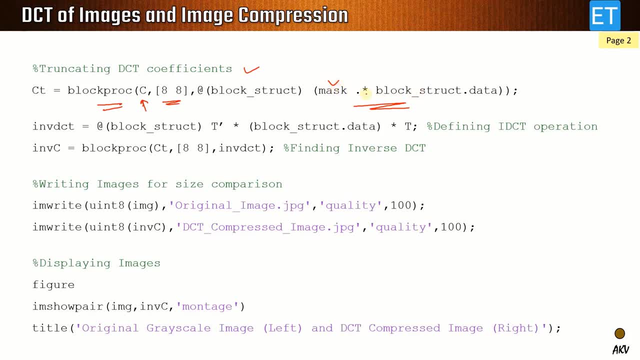 in this operation. you can simply see that mask is simply multiplied element by element with that block of 8 by 8 DCT coefficients. So by multiplying this mask, obviously your top left corner- few coefficients will be preserved and then rest will be made 0. So now we have to take the inverse. 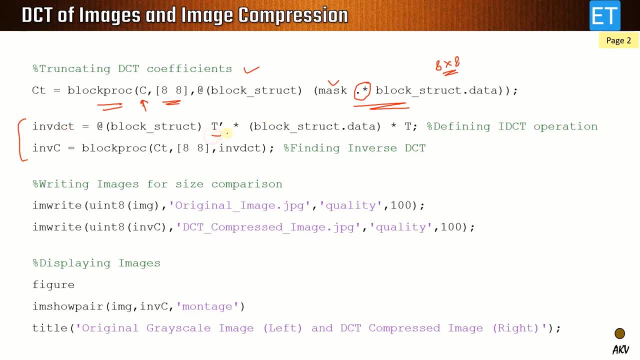 transform. So we are defining the inverse transform. again, There is the T transpose and then 8 by 8 block, and then T matrix, and then doing this operation on all blocks of your image. So here in C, in INBC, you get your image, which is, which is compressed, actually by neglecting various 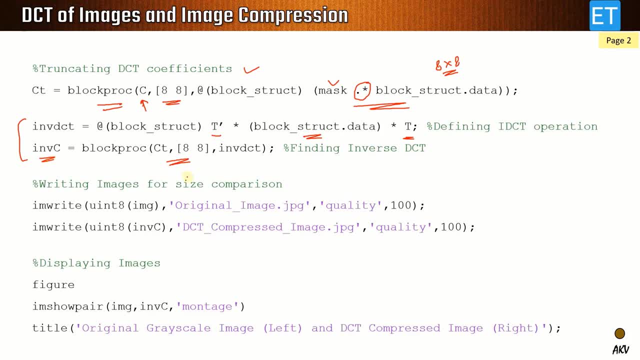 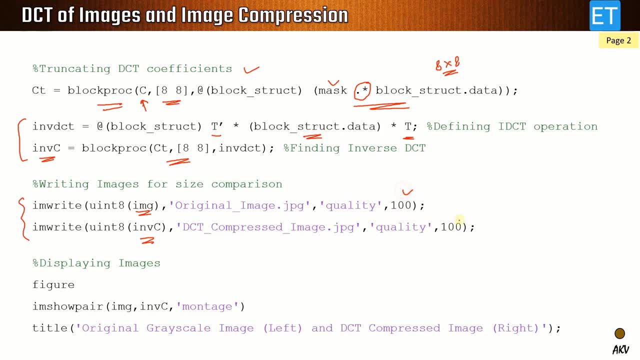 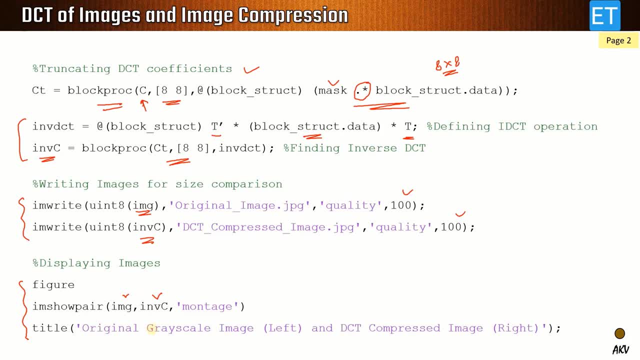 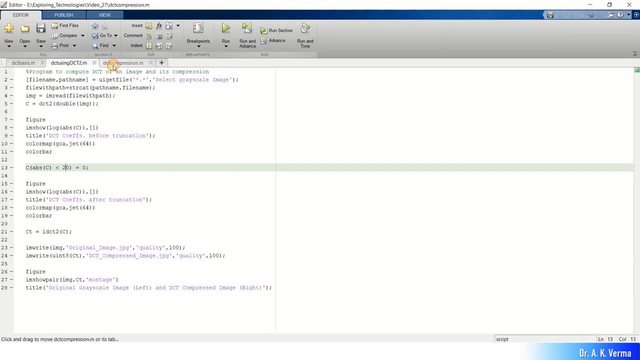 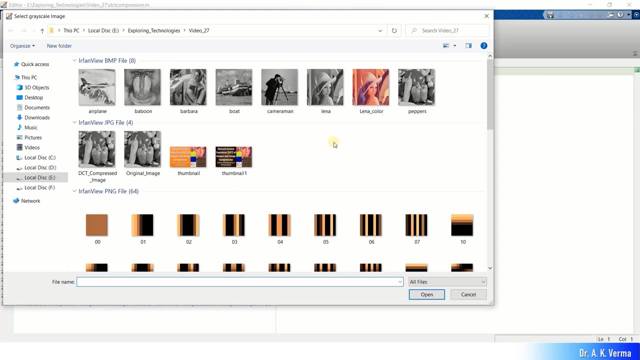 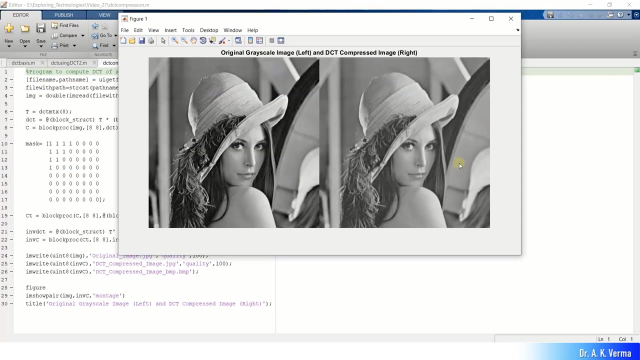 comparison. So let me run this program in the MATLAB so we can have the better idea. So, just opening this in editor and this program is already written. So I'm just pressing this run button. Okay, so it is asking me to choose my image. Let I am choosing this, Lena, And let's see what output I achieve, So you can see. 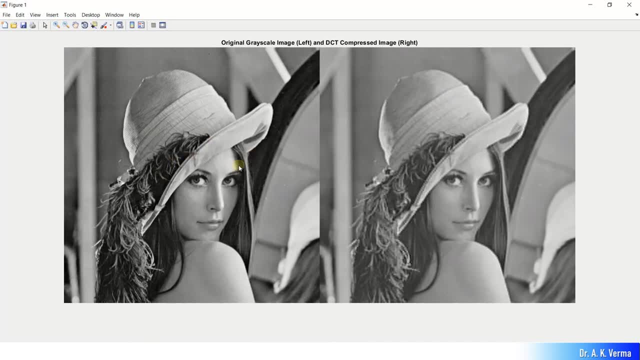 this, these two images. So this one is your original image and this is your DCT compressed image. So, quality wise, there is not not much difference. There is a slight blur actually in this image because- and that is natural- because we have neglected all the high. 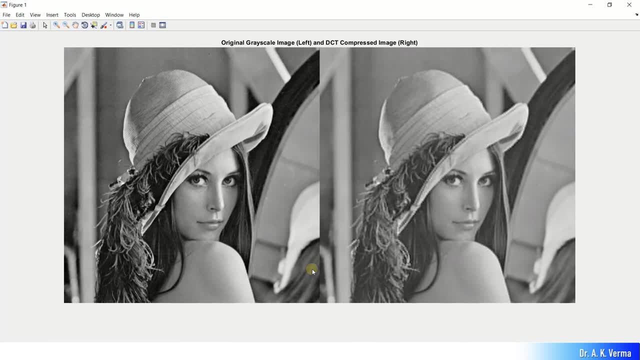 frequency components I mean we have, although we have kept few at the top left corner, but we have neglected most of the high frequency components. So obviously the blurring will be achieved. So no surprise, but it's still. this quality is acceptable. Okay. So now let me see the